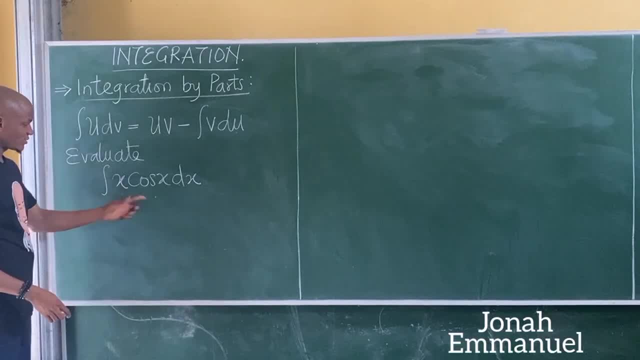 Alright for this. now this x cos x- here's the x, So I'm integrating this with respect to x. x becomes my integral variable. So to solve this now, what I do is this: Relate x cos x to what I have here. 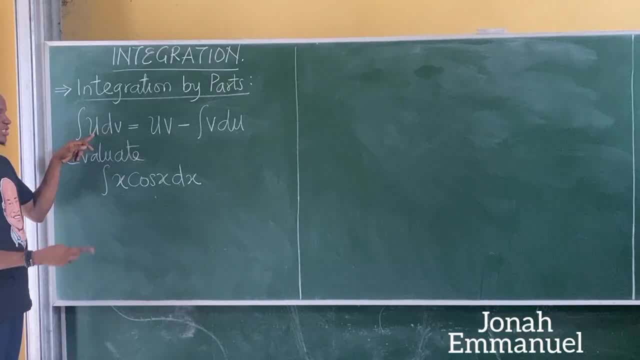 That means u. this is u multiplying dv, This is x multiplying cos x. So obviously, if I should match them up, u becomes x and then dv becomes cos x. So for this I will say: let's u be equal to the first one here, that's x. 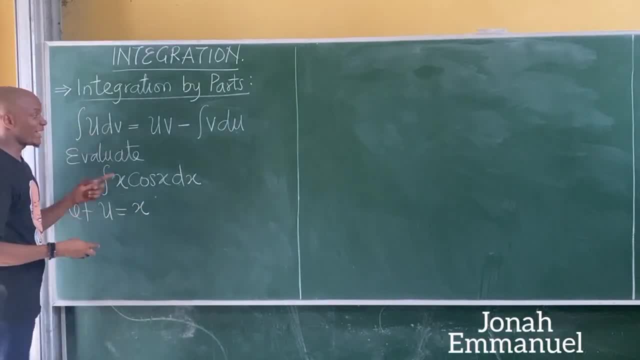 And also notice that u is multiplying dv and not just v. So if u is x, it means that dv equal to cos x. So also let's dv equal to cos x. If I cross u to get the value of du, I will have to differentiate. 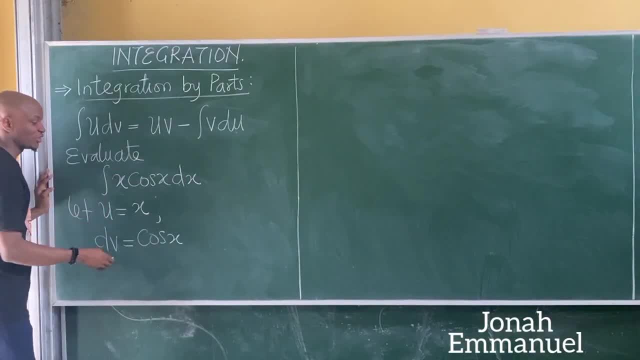 So, hence, if u is equal to cos x, I will have to differentiate. If I differentiate, I will have that du is equal to y. So if I differentiate x, I get y. Also, if I have that dv is equal to cos x, to get the value of v I will have to integrate. 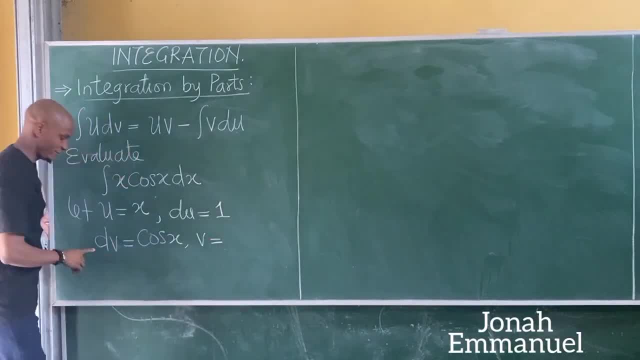 Hence, if I integrate dv, I will get v, If I integrate cos x, I will get sin x. So I've got my four major parameters, That's u, which is x, du, which is 1, dv, which is cos x, and then v, which is sin x. 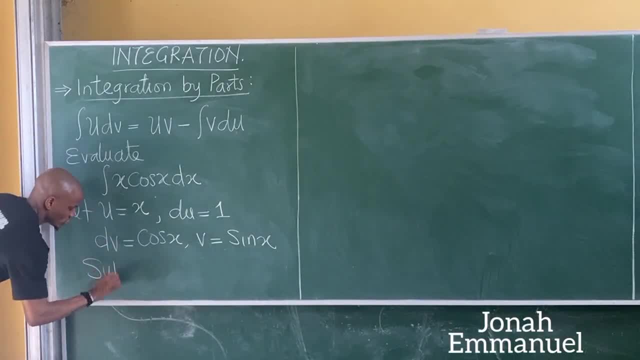 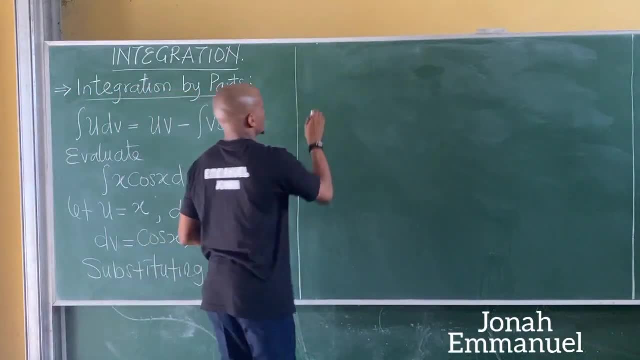 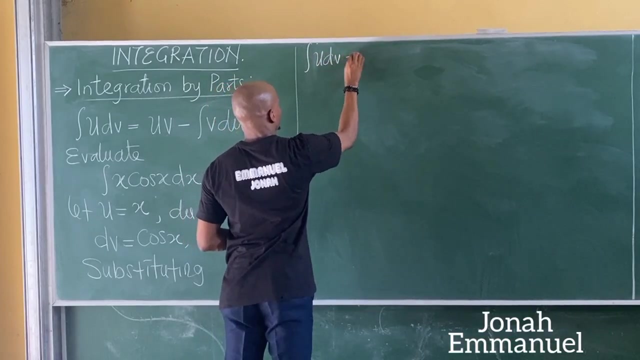 Alright, next up now I will substitute. So, substituting, I will substitute these values into my equation. Substituting, I have that the integral u dv is equal to uv. Subtuting, I have that the integral u dv is equal to uv. 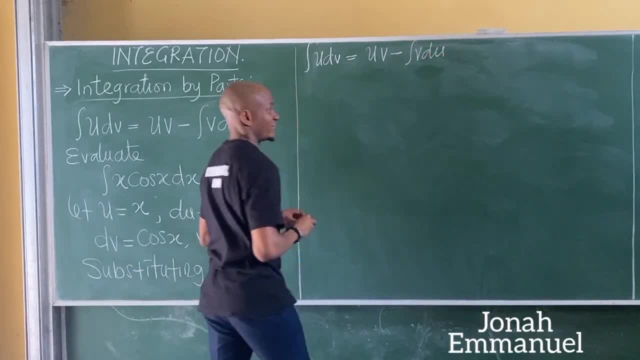 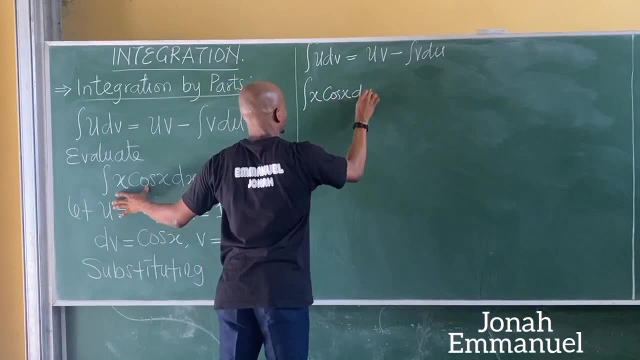 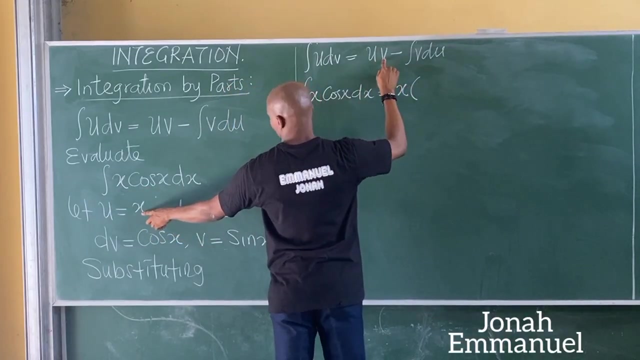 Minus integral v du. So I have this. Alright, repeat the question Here. I have that the integral u is cos x. cos x dx is equal to uv u. here is what u is x. We call this x there Into v. 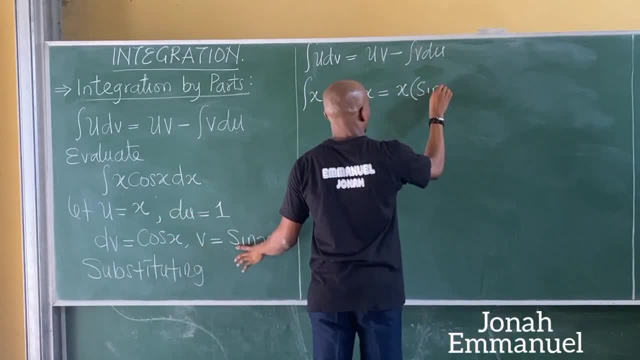 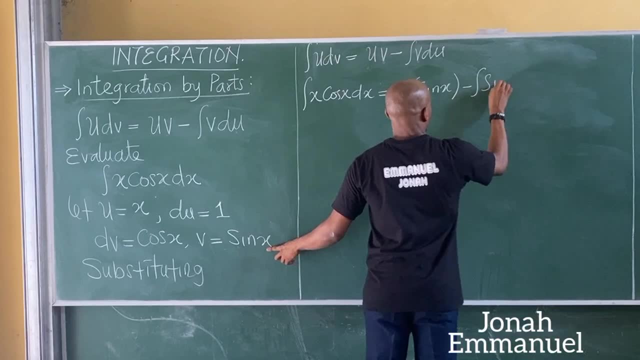 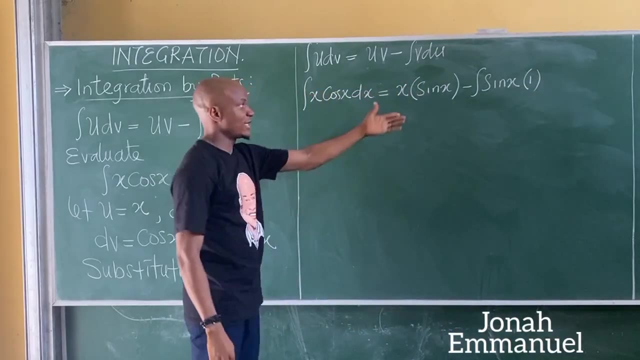 v is sin x's value, So x sin x minus the integral of v, v in value is sin x. So sin x into du, du in value is 1.. So I'm having 1 here, Alright. so this is after substituting. 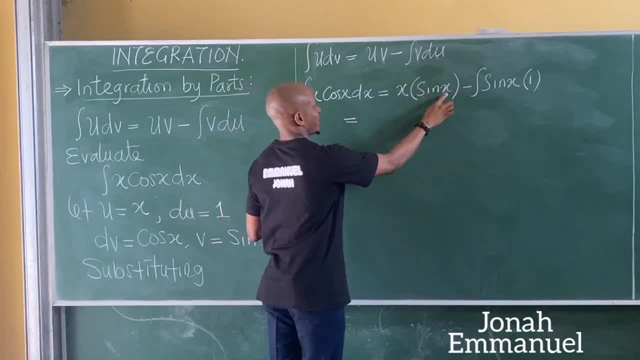 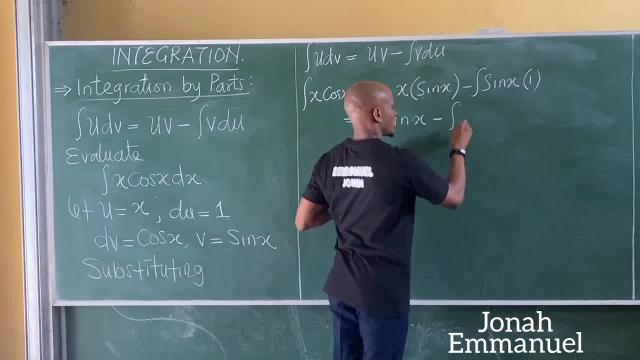 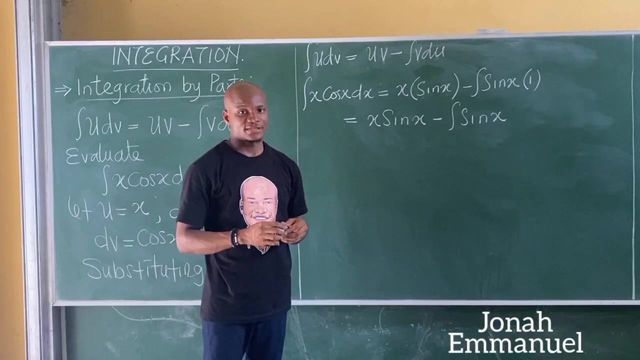 If I work on this, it will now be equal to x times sin x gives you x sin x minus the integral sin x times 1 gives you sin x. So I'm having x sin x minus integral sin x as my result of this. 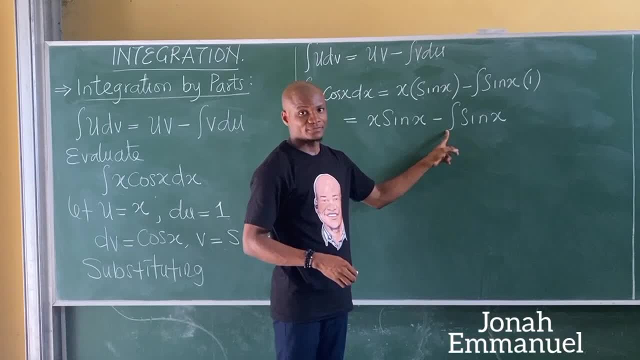 But I will not stop here because I'm sitting at the integral sin, Hence I will have to evaluate this integral Now. also note that when it comes to evaluating this, I am integrating sin x with respect to the same integral variable here, which is actually the x. 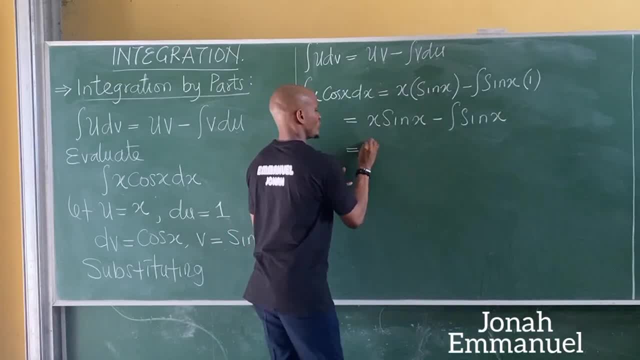 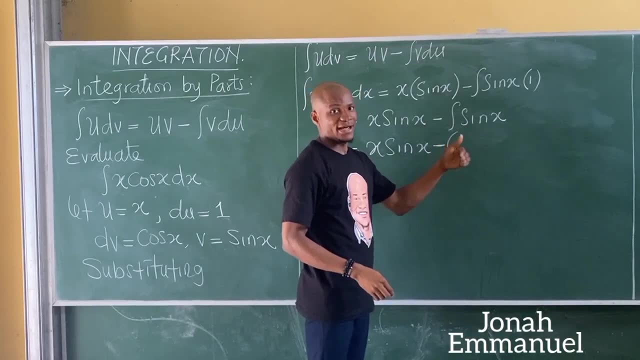 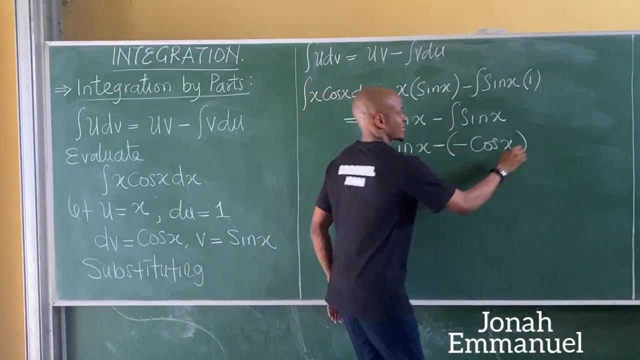 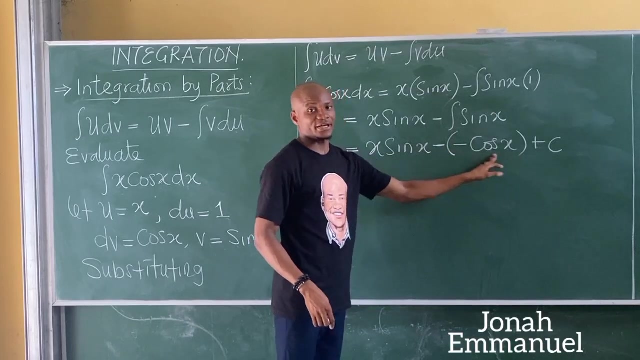 Alright, such that this now becomes equal to x sin x minus. if I integrate sin x, I get minus cos x. It becomes minus cos x, Alright, of course, plus c, which is the constant of integration, because after doing my final integration here, there is no more integral sin here. 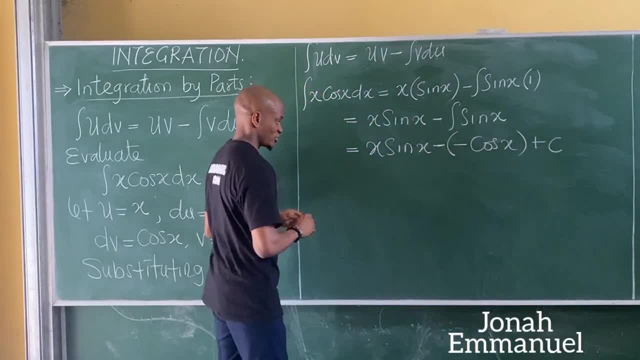 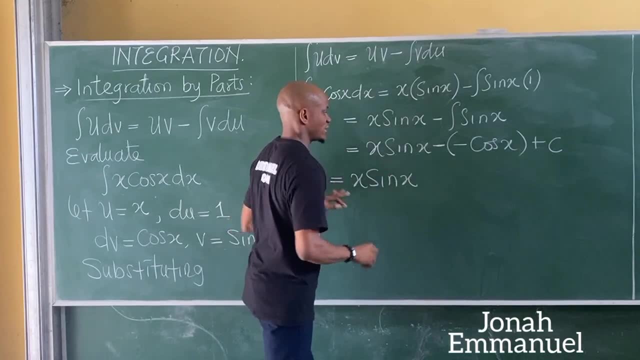 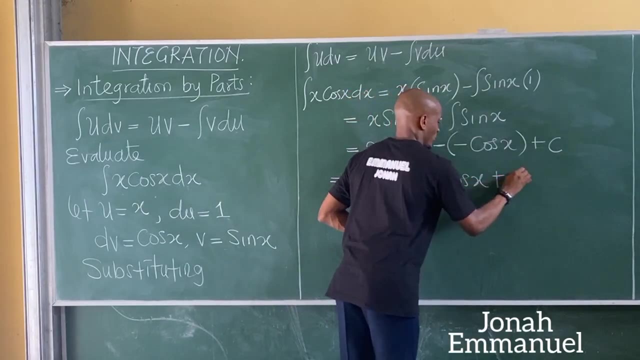 So you now put plus your constant of integration Work on this. This is now equal to x times sin x gives you x. sin x Next up. minus. minus gives you plus Next up. loving cos x Next up plus c. 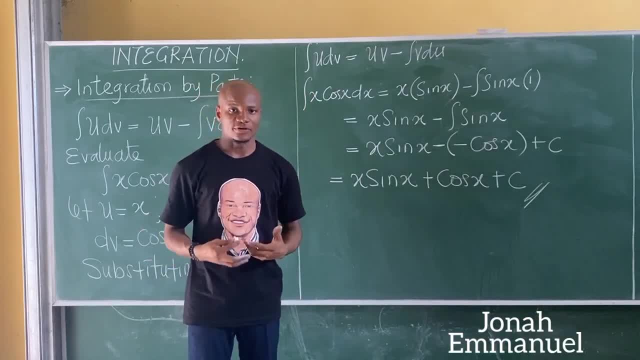 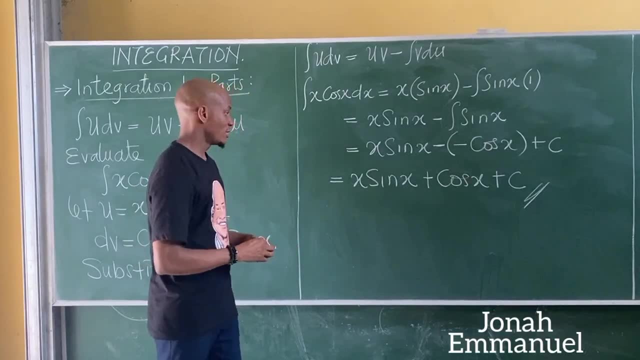 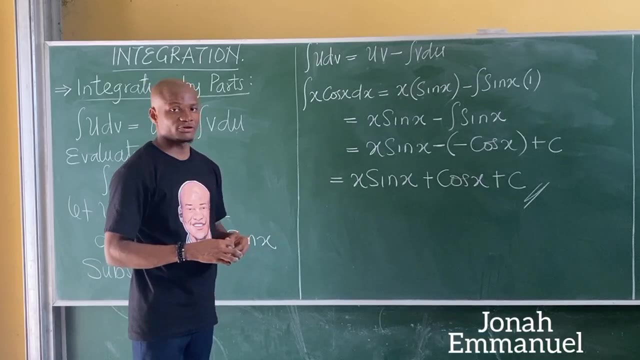 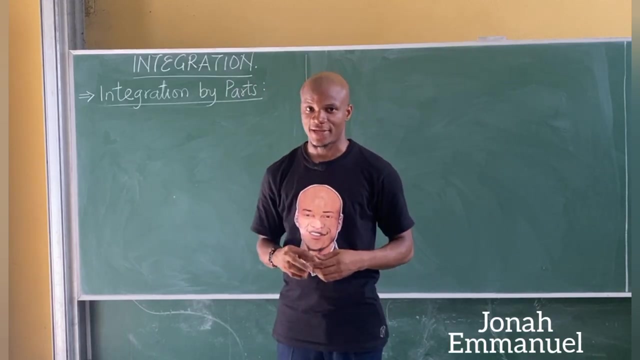 So this is how you work on terms using integration by parts. So my answer becomes x sin, x plus x, cos, x plus c. So that's like the result after using integration by parts. So take a second example on integration by parts, But before then, 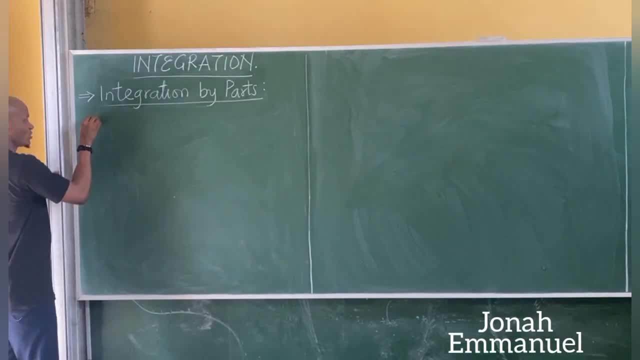 let's first start this example. Let's say we ask to integrate exponential 3x, Something like this, Obviously with respect to the x. If I should work on this now For this case, I have to use integration by substitution for this case. 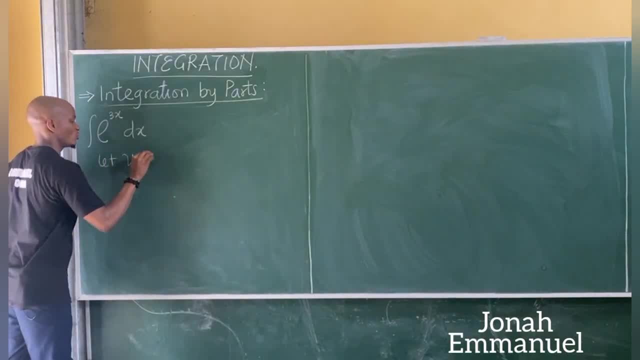 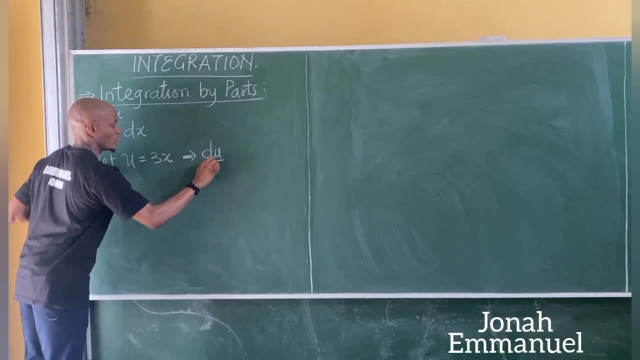 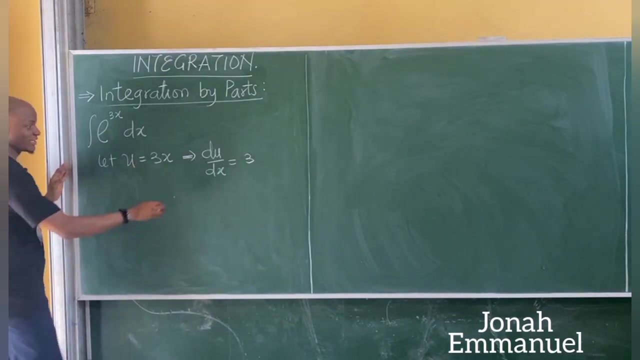 For this I will say: let u be equal to 3x, Such that if I differentiate I will have that du all over the x Is equal to 3.. After differentiating this, Such that the x- The x here- is equal to du all over 3.. 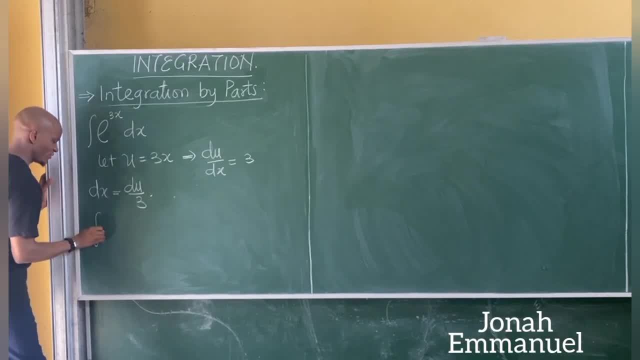 And also I will now have that the integral exponential 3x. The x is now equal to the integral exponential With respect to 3x equal to u. This becomes u, dot, dx. The x in value is du all over 3.. 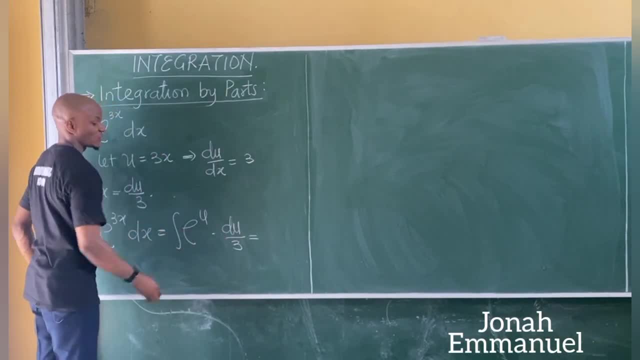 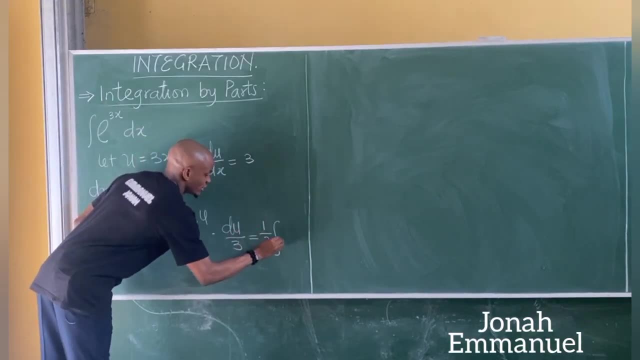 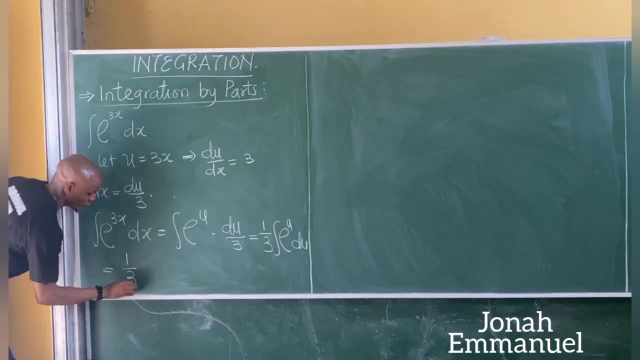 From here now. my constant here is 1 over 3.. So take the constant outside the integral side. It becomes 1 over 3. integral exponential u du. Alright, so this now becomes equal to 1 all over 3.. If I integrate exponential u du. 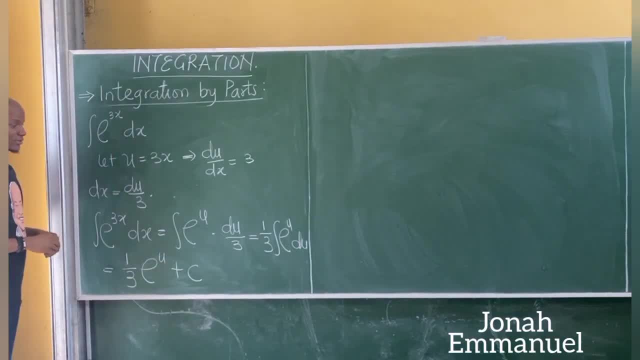 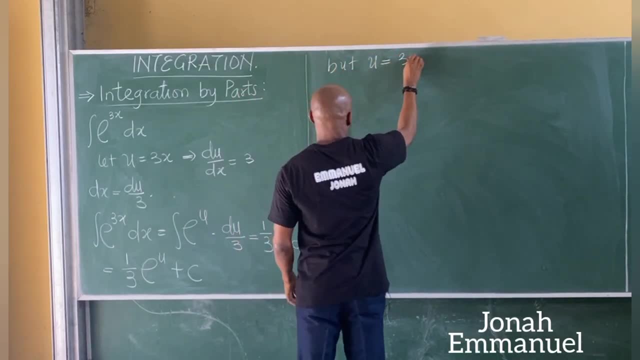 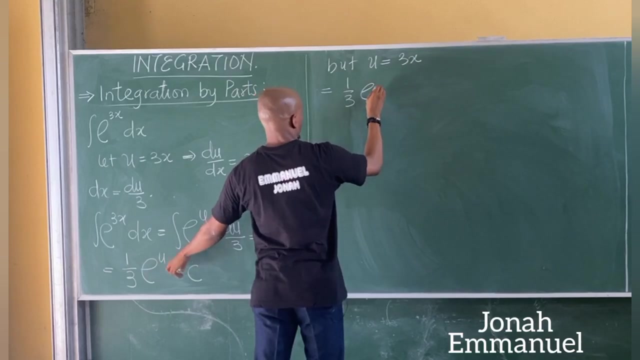 I will now have exponential u plus c From here. But we said u is equal to 3x, So my value now is equal to 1 over 3.. Exponential u u in value is 3x, Then plus c. 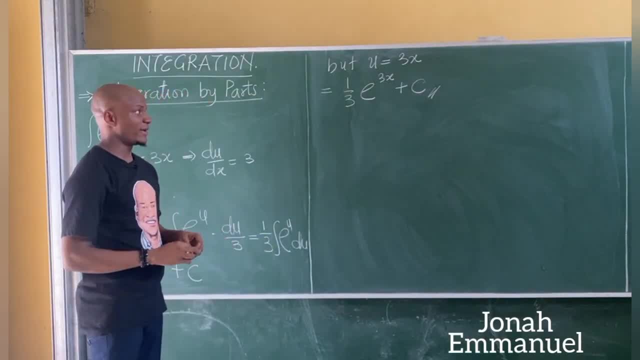 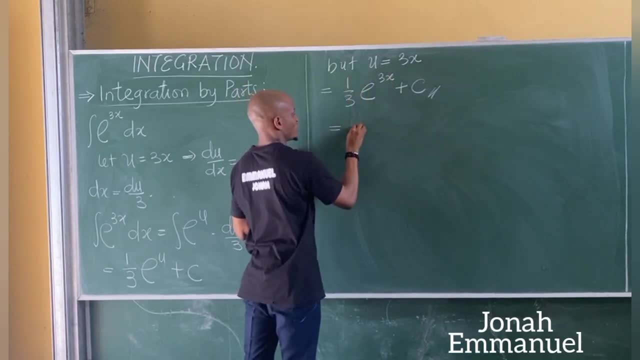 So I have it as my answer. You can also rewrite it as saying: this is equal to 1 over 3 times. This gives you Exponential 3x times 1, gives you Exponential 3x- all over 3 plus c. 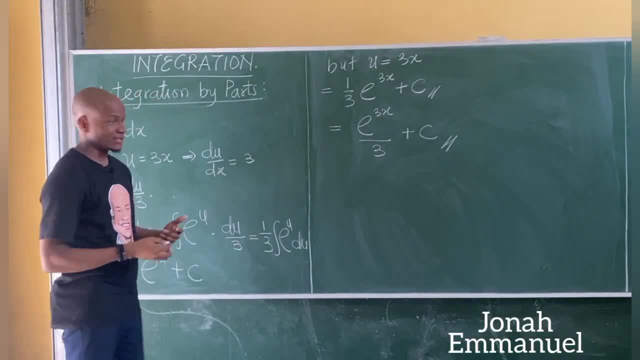 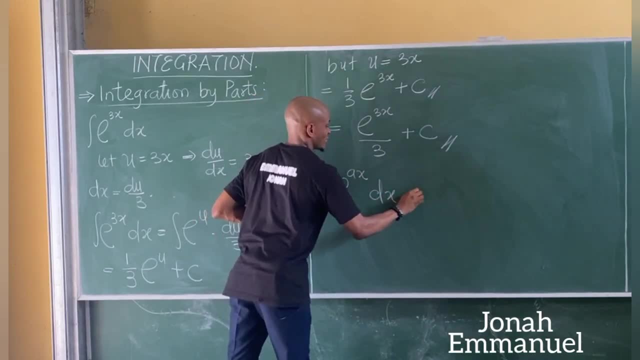 So I have this value. The concept is this: If I am asked to integrate the exponential of a pen With respect to the x, My final answer becomes the inverse of this term. here, Of course, if I differentiate ax, I will be left with a. 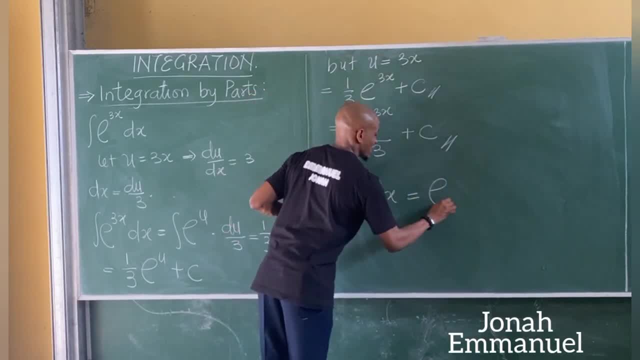 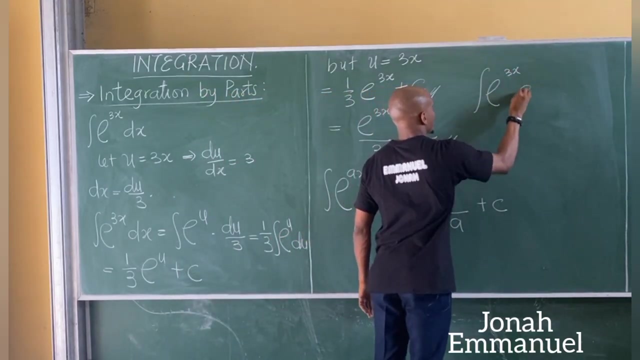 So the short course is this: Simply repeat this Thus: exponential ax all over. Differentiate the part. If I differentiate the part here, It gives me a Then rc. That is like a simple concept here, Such that if I am asked to integrate exponential 3x dx. 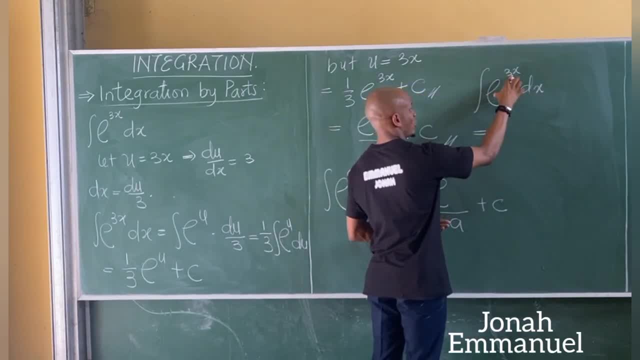 My final answer is easy. What you do is this: Repeat this math Or write this math here. It becomes exponential 3x. all over, Differentiate 3x, It gives you 3.. I must see, And this was the answer there. 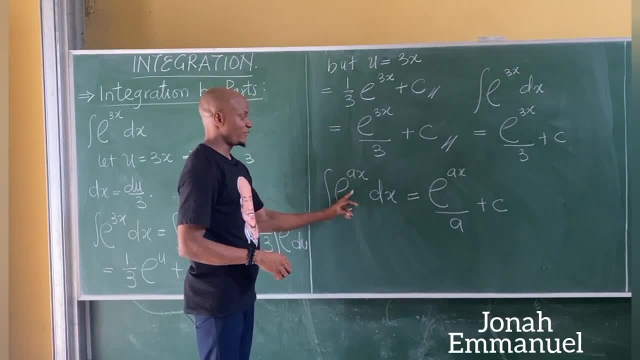 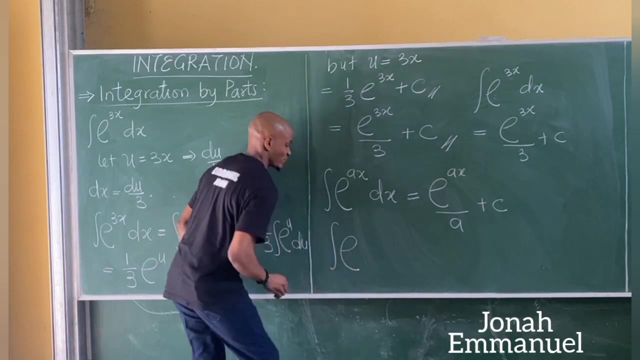 So the short course of integrating terms involving exponential Is simply to write down this term as your numerator All over, Differentiate the index or this part And keep it as your denominator. One last example, If I am asked to integrate exponential: 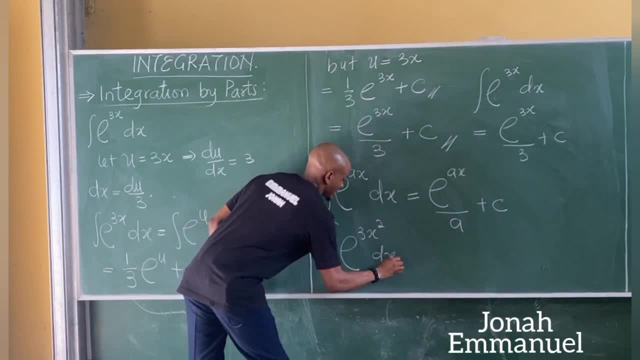 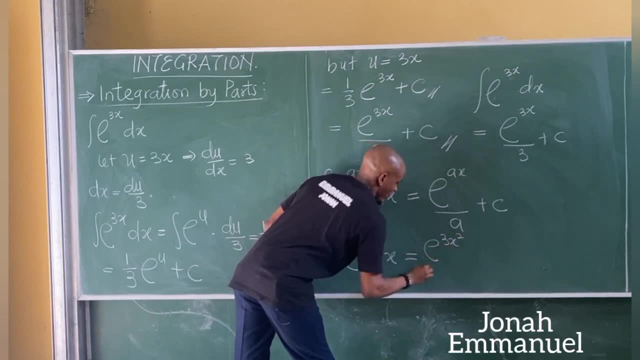 Let's say 3x square dx. This will be equal to Write down this term. This term is exponential: 3x square, All over. Differentiate 3x square, You get 6x. So all over 6x. 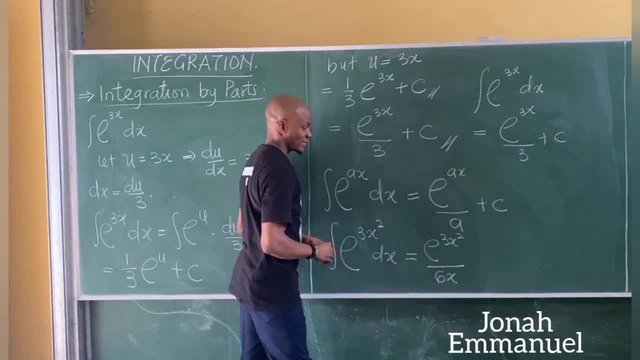 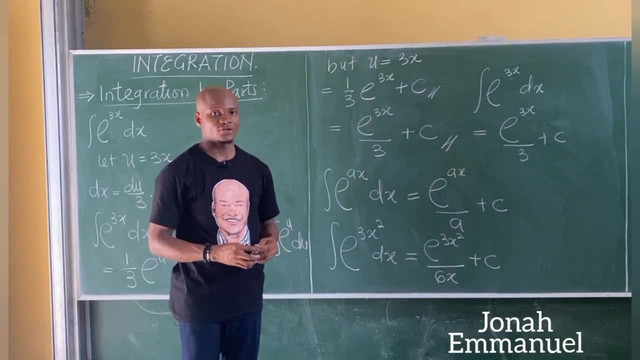 And of course, Plus c. So this becomes like The answer to This question. So this is like a short course On how to Integrate Exponential Functions. So let's look at How we can actually use. 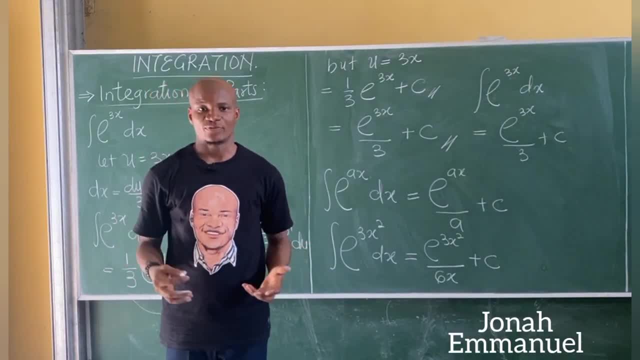 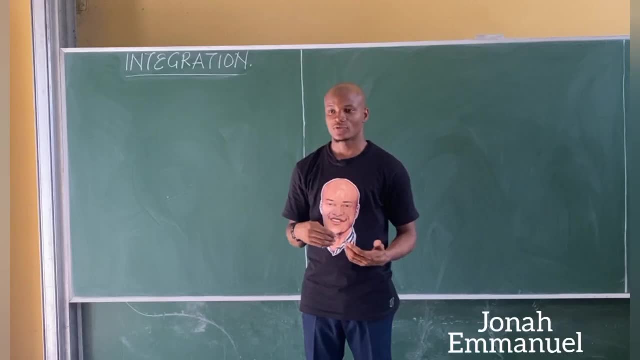 The short course I just showed you How to Integrate Exponential Functions. So let's look at How we can actually Use The short course I just showed you To solving problems On integration, For instance. 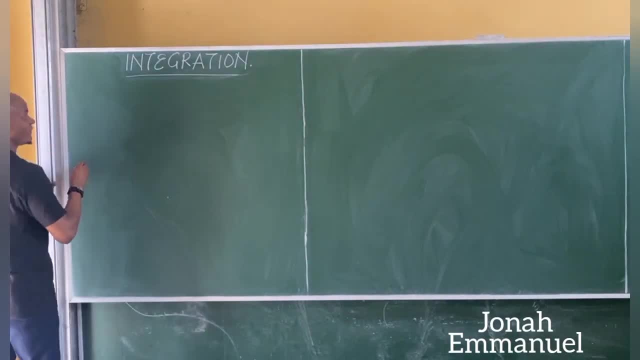 Let's say We are asked to Evaluate The integral Of X square Exponential 3x, dx. All right, So let's say We are asked to Evaluate This integral. What do we do For this case? 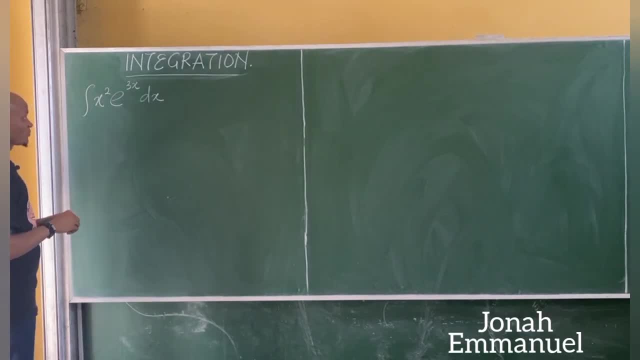 Remember that Our formula is: Integral Of u dv Is equal to uv Minus Integral Of v du. All right, So for this now I'll call this u, So Let u. 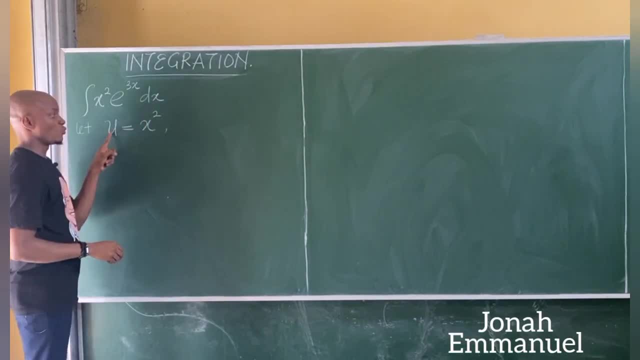 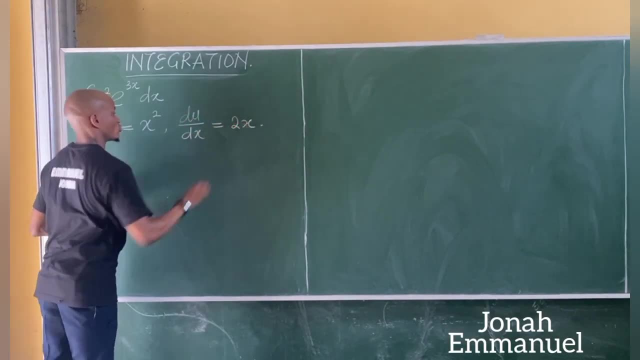 Be equal to What I have here: X square, Differentiate u With respect to x. I'll guess that du All over dx Is equal to 2x. Next up I will say: Let v. 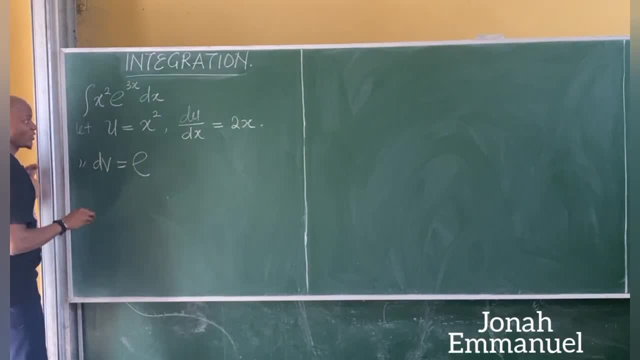 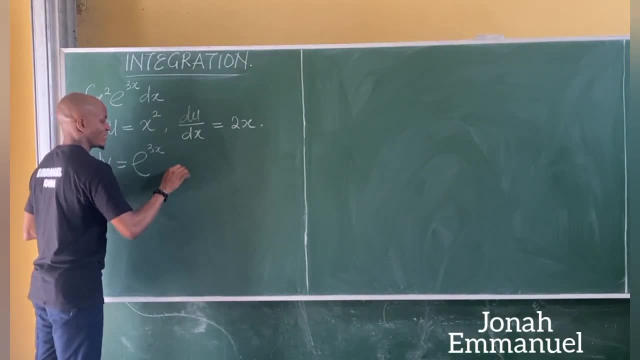 Be equal to x, Or let v Rather Be equal to Exponential 3x. From here I'll have that v Is equal to Repeat this, That's Exponential 3x. 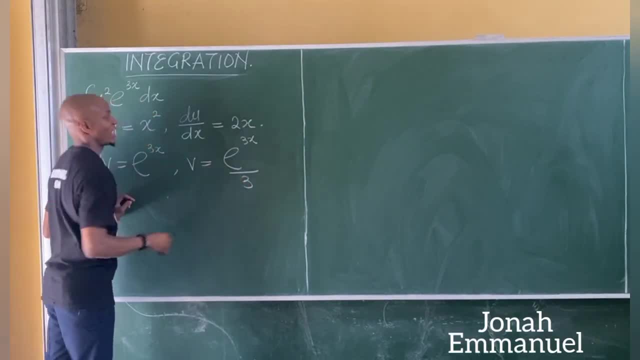 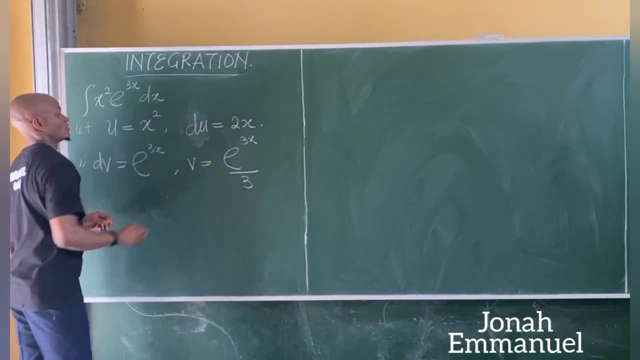 All over. Differentiate 3x, I'll guess 3.. So I have this one here. Perhaps We can take this as du Instead of du x. This is my du value, So Substituting. 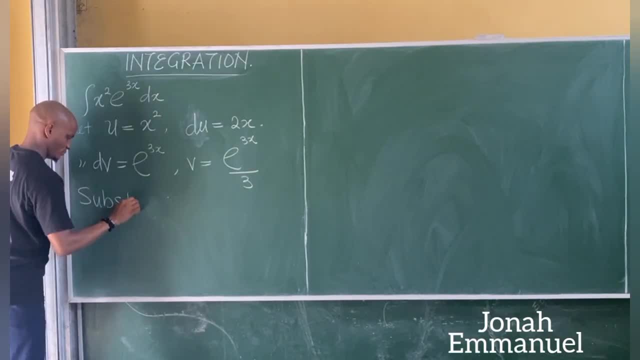 Into Substituting Into This Value Of x Into The value Into The Integration By Part Formula, I have that The Integral u The v Is equal to. 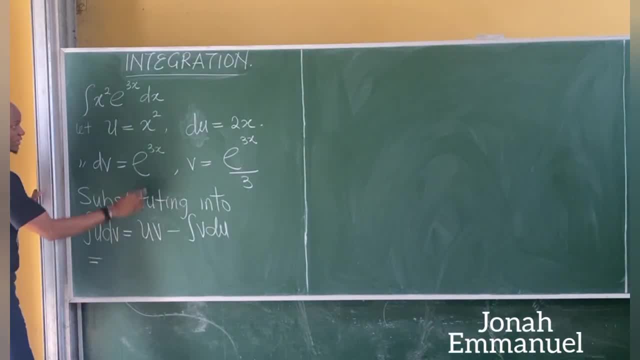 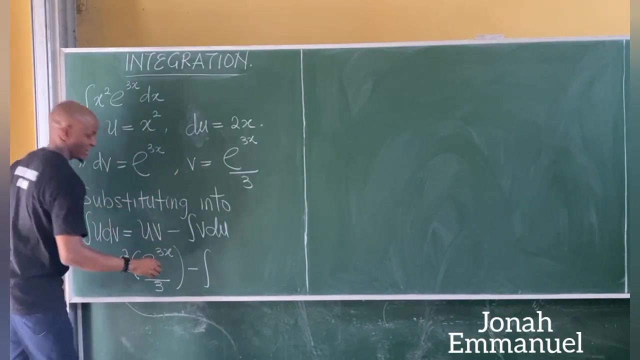 u v. Minus Integral v Du. All right, That's Now Equal to. u Is All Over 3. Minus Integral v v- Yes, Exponential 3x. 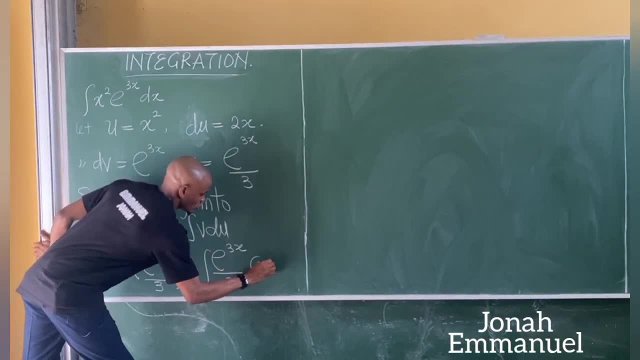 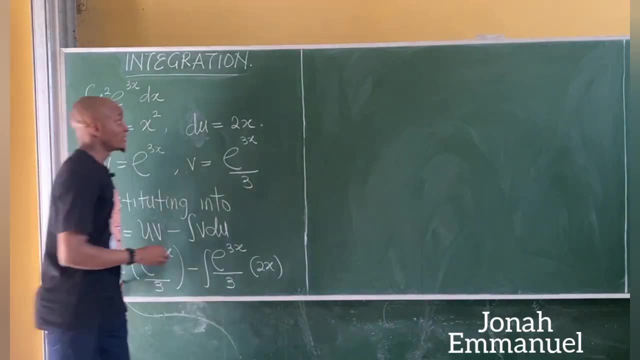 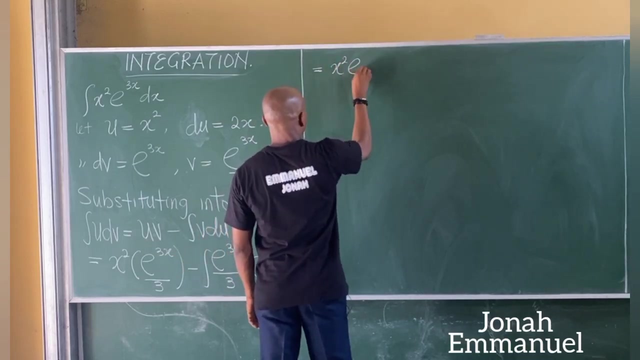 All Over 3.. Into du du Get Is 2x, So I have This Value. You Have To Work On This. 3x. All Over 3.. 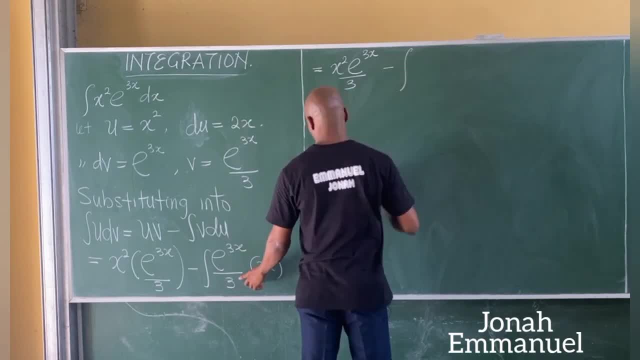 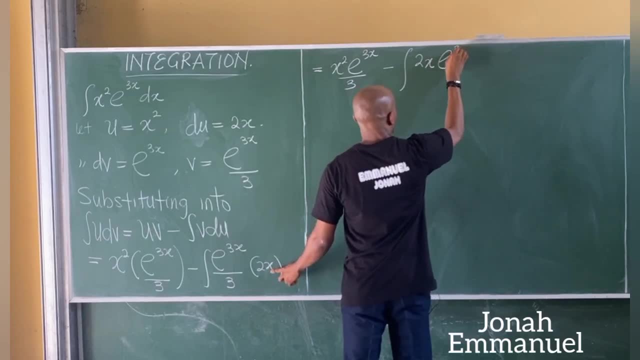 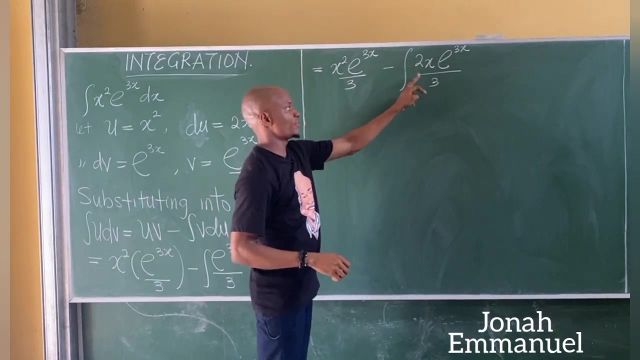 Minus, Minus. I'm Having This As Integral, So This Was Playing This Issue 2x, Exponential 3x, All Over 3.. So I 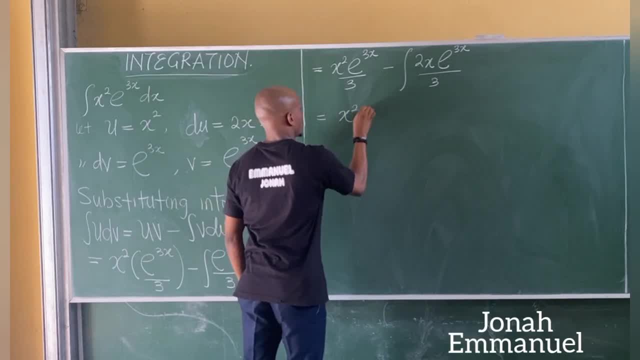 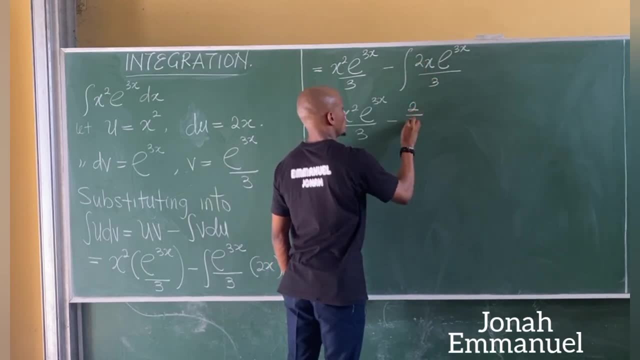 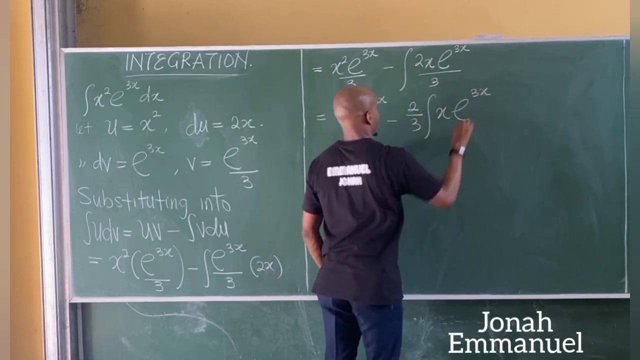 Have This, So The Exponential 3x All Over 3.. Minus This Is 2. Over 3.. To Take Out: 2. All Over 3.. 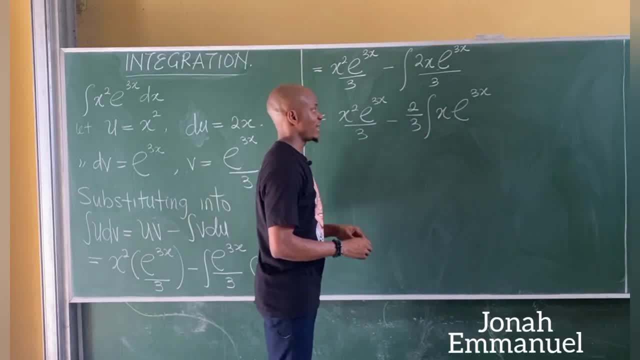 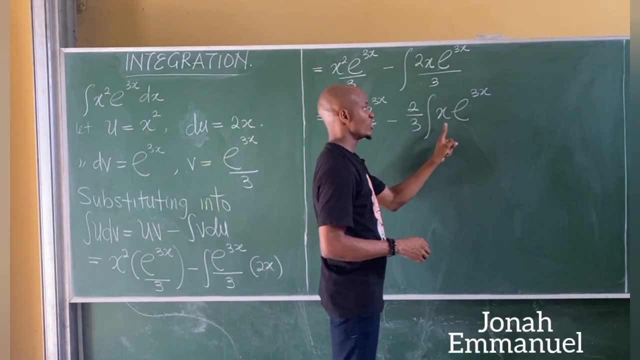 Integral. I'm Left With X Exponential 3x, If I Take Out. This Is Still In The Form Of Integration By Parts, So I Will. 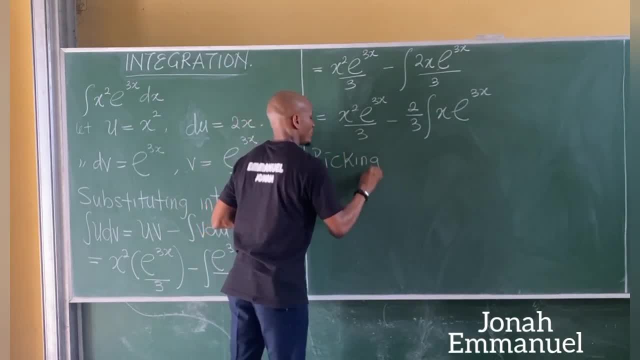 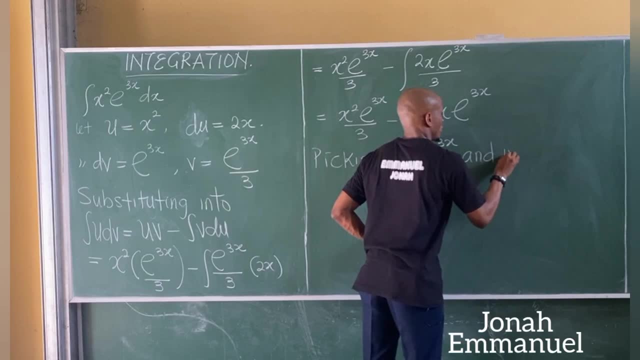 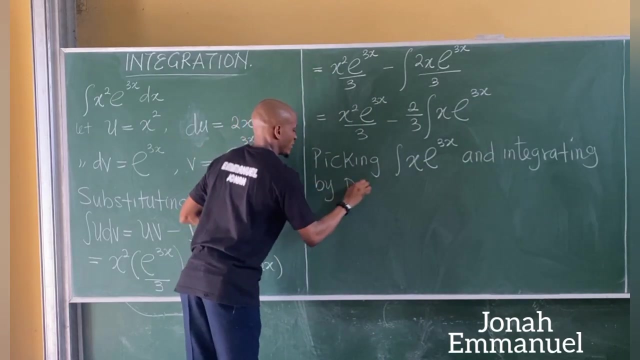 Perform Another Operation On Integration By Parts Using This. So In This Case Now My New Five Parts. I Have That For This. The Integral X. 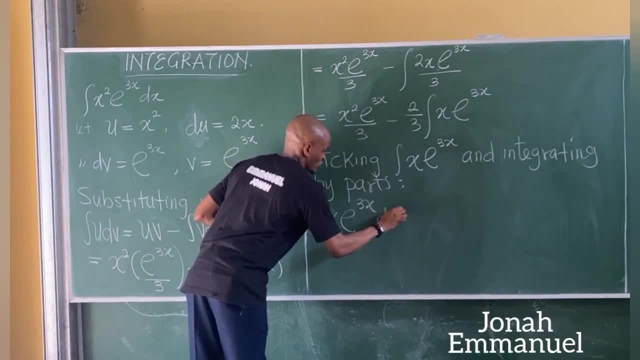 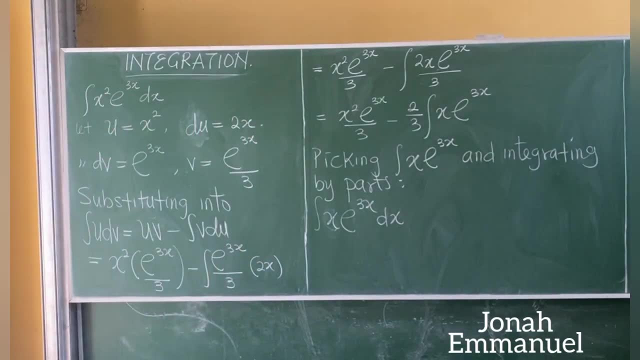 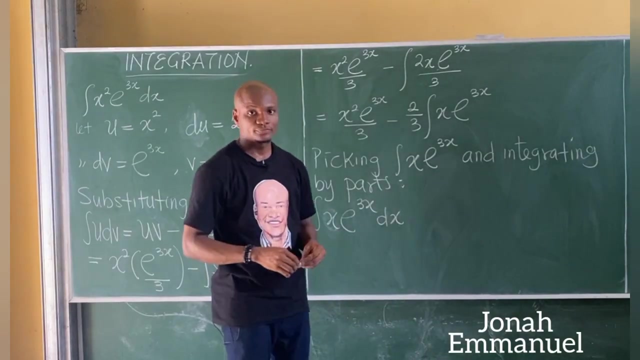 X, Exponential 3x For This. Of Course, With Respect To X, That X Is My Integral Variable, So I Have So For This Now. 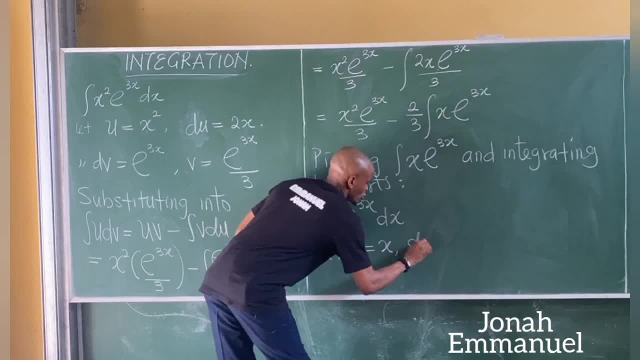 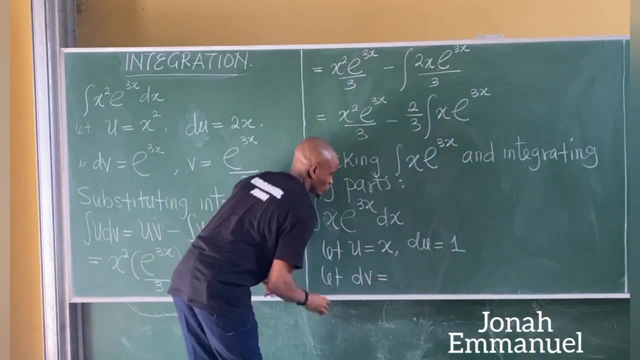 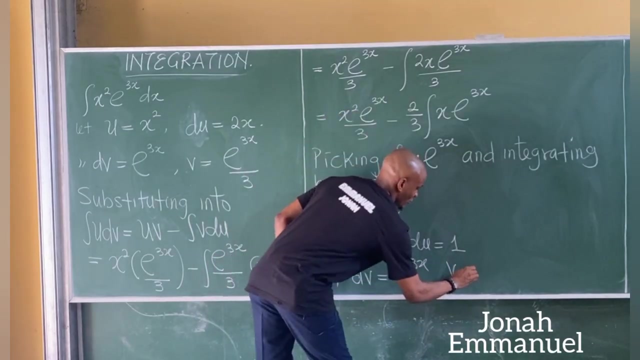 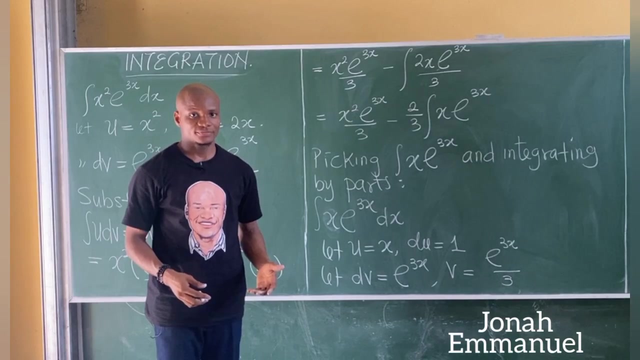 Let You, For This Case, Let You Be What I Have Here: X, Such That The You Is Equal To One. Also, Let The So Take. 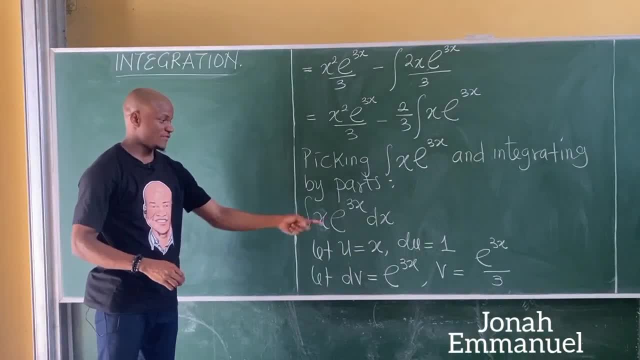 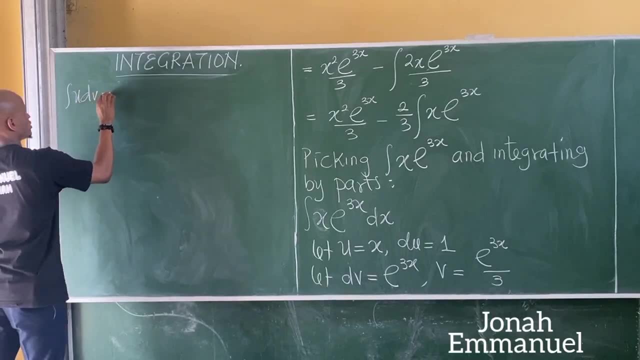 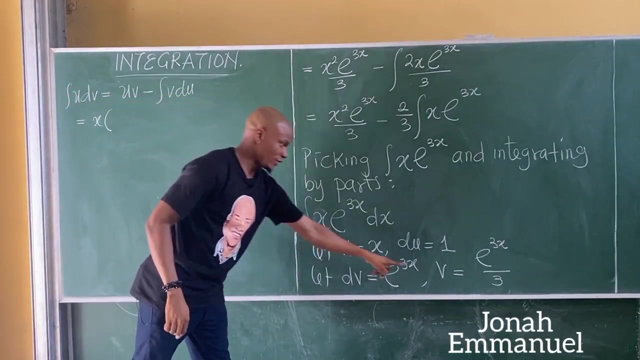 This Off. So If I This, I Have That. We Said The Integral You, The V, Is Equal To You. So This Now Be Equal To. 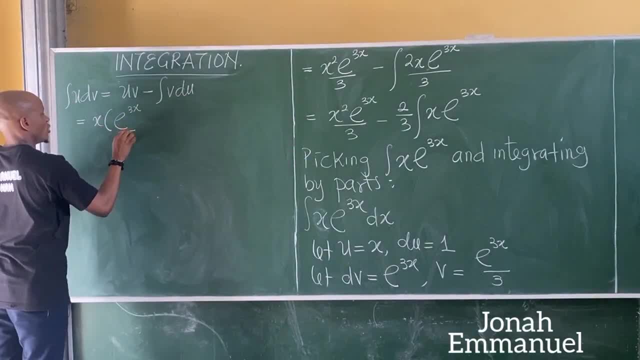 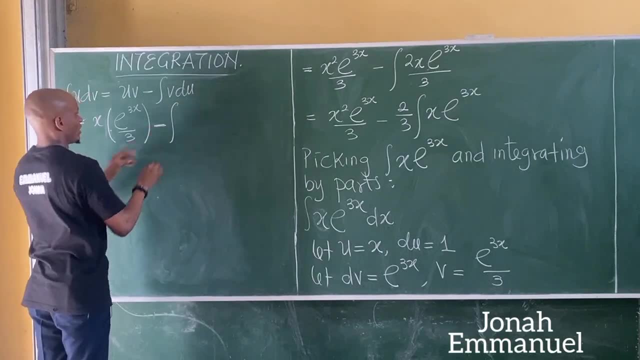 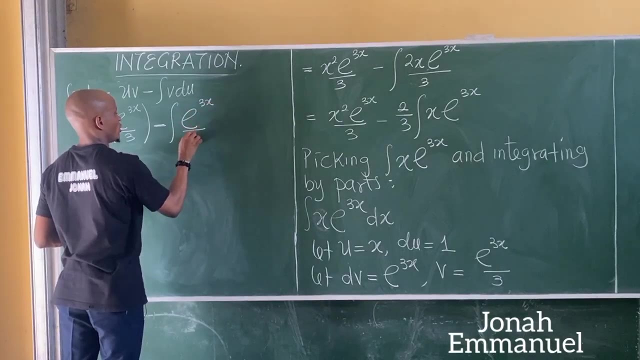 You Exponential Three X All Over Three Minus, Minus The Integral V, V In Value, Is This Exponential Three X All Over Three Times. 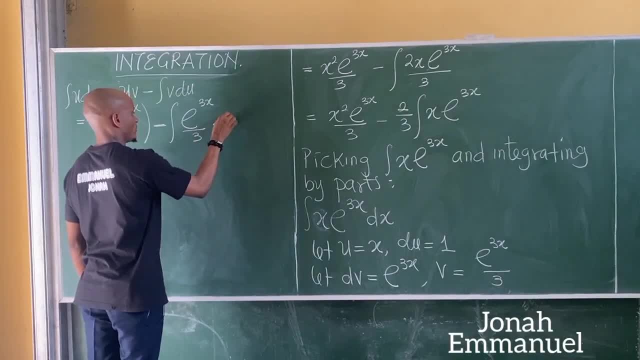 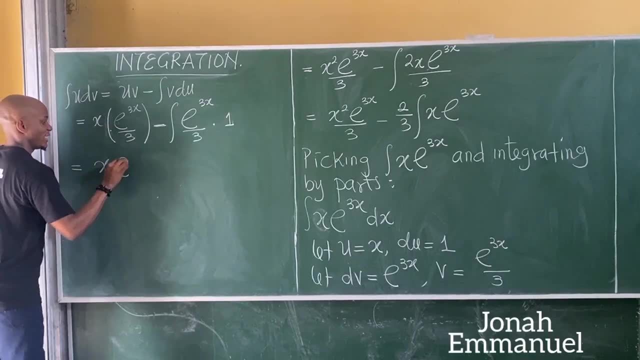 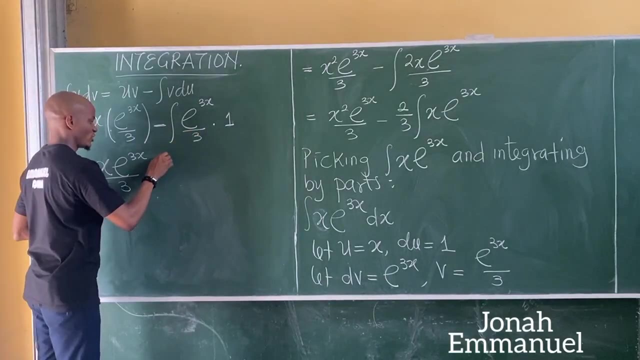 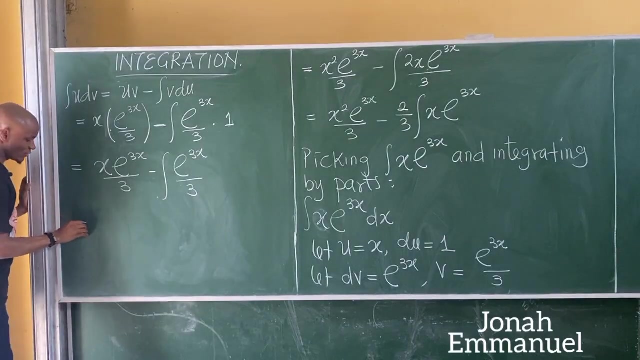 The You. The You In Value Is Now Equal To X Times. This Gives You X Exponential Three X All Over, Three Minus This Times. 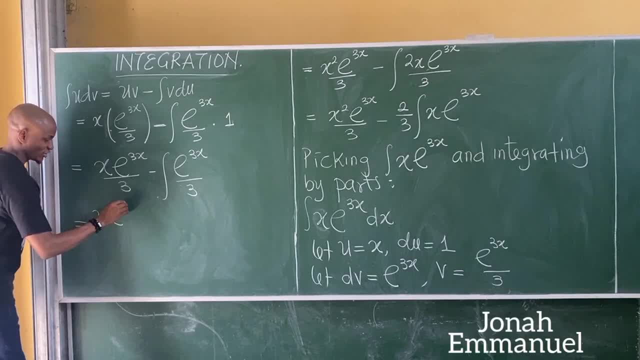 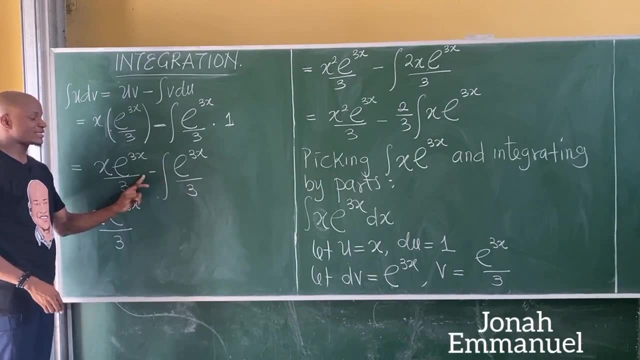 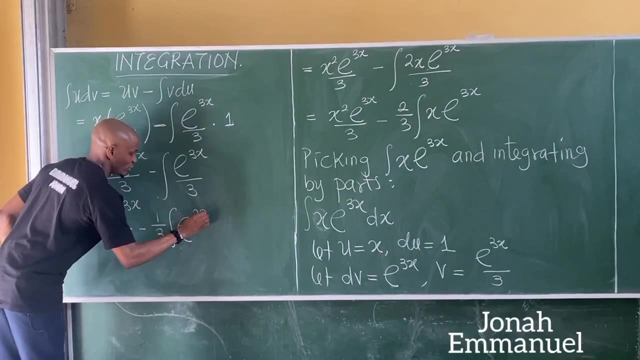 One Gives You Itself. So Becomes Integral Exponential Three: X All Over X. Becomes Minus One: All Over Three Integral Exponential Three X. 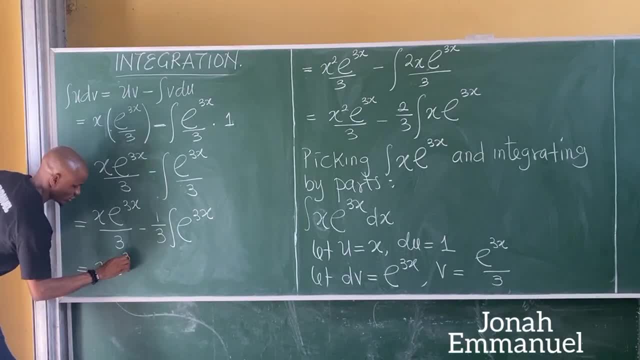 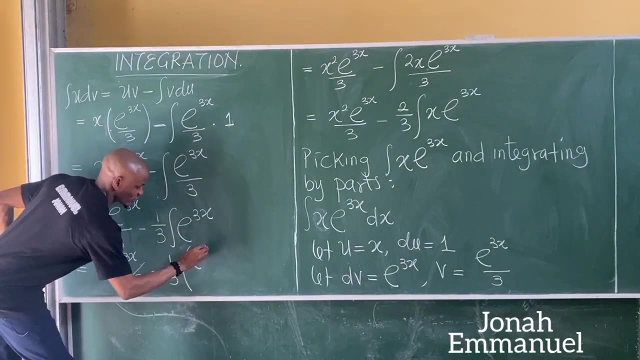 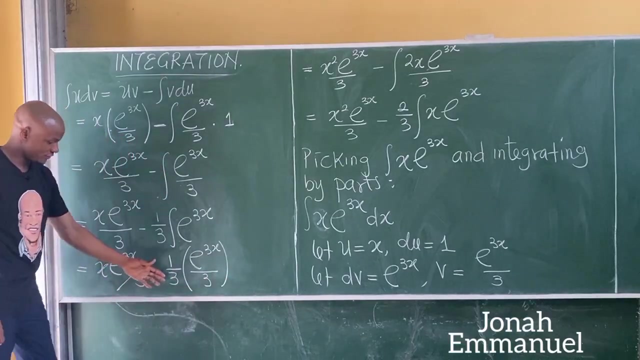 So I Can See Evaluate This. This Is Now Equal To X Exponential Three X This All Over Integral, Three X All Over Integral. If. 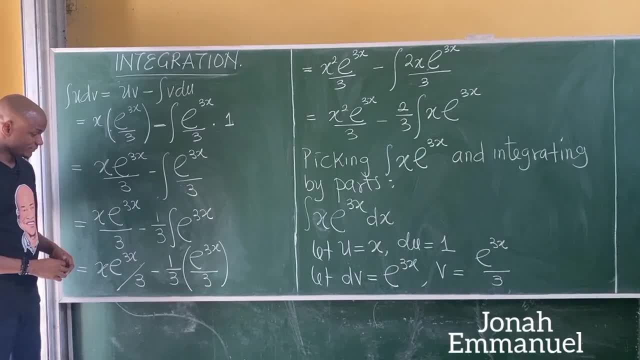 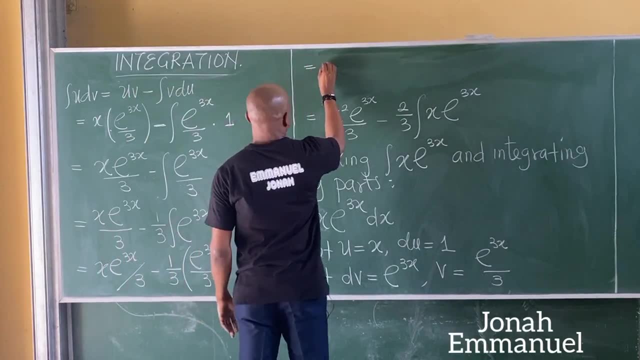 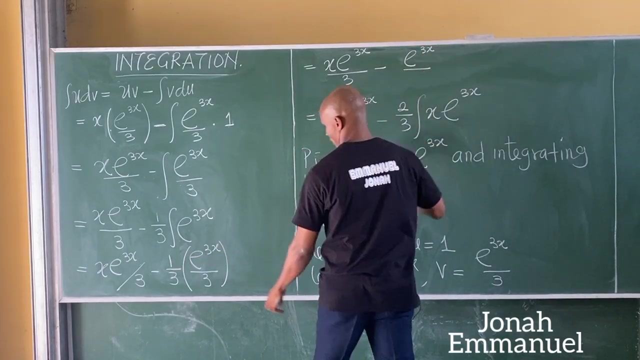 I Shape This Against The Such That This Now Gives You A Value Of Like Nine. Okay, Now, Here's The Thing. So I Have Three. 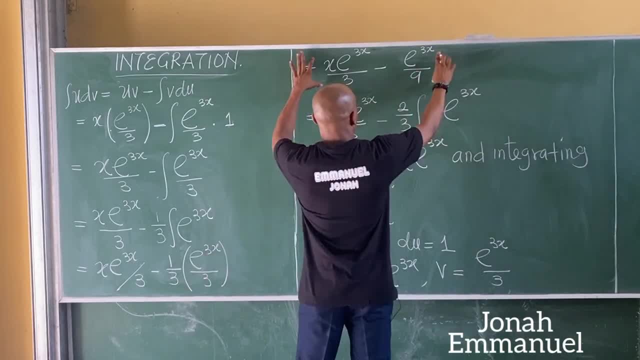 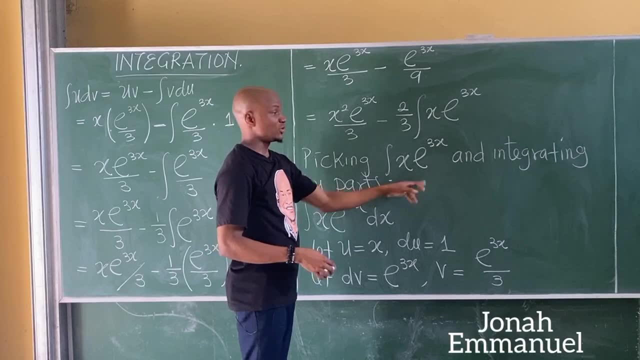 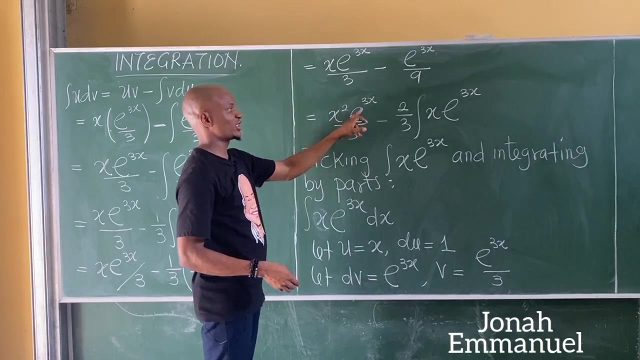 X. All Over, Three Times Three Gives You Nine. All Right, So This Value, This Value Is My Final Answer After Evaluating This Integral. So 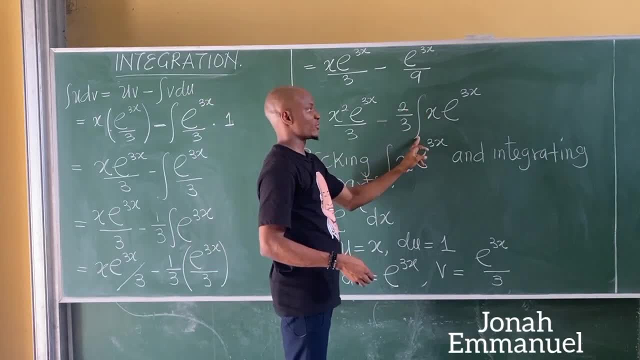 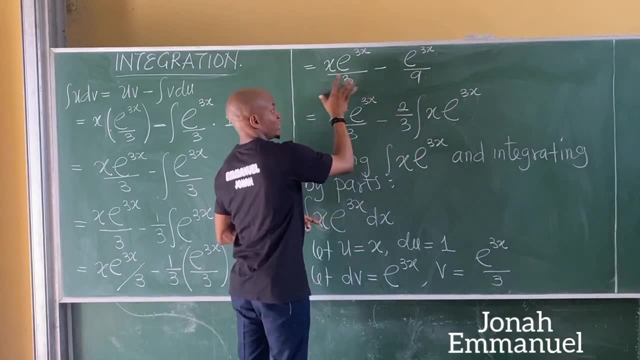 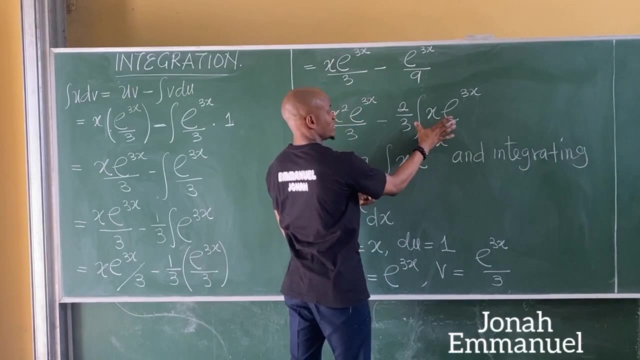 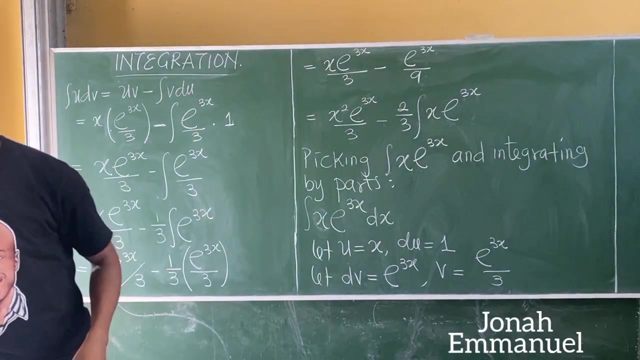 The Value Minus Two By Three Integral. This Now The Value For The Integral X Exponential Three X. This Value Is Now Equal To This. 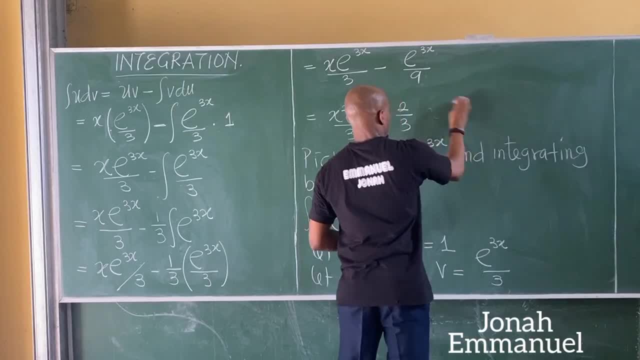 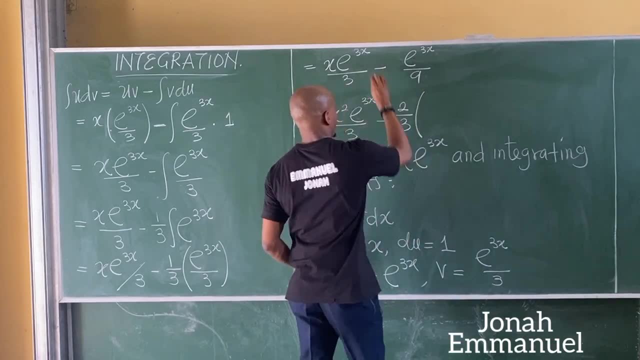 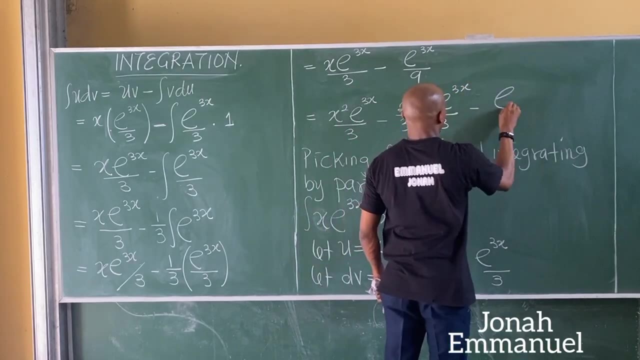 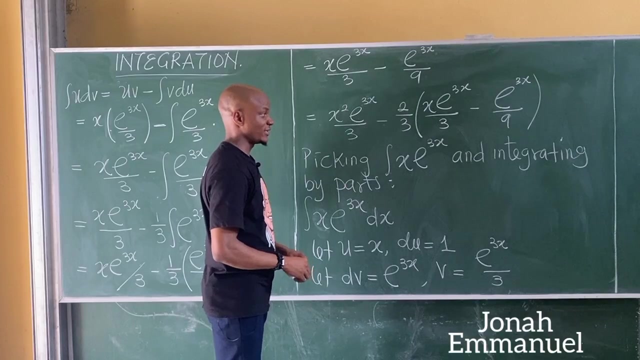 So In This Case Now, In Place Of That Integral X Exponential Three X, I Will Not Have This Value. Thus X Exponential Three X. 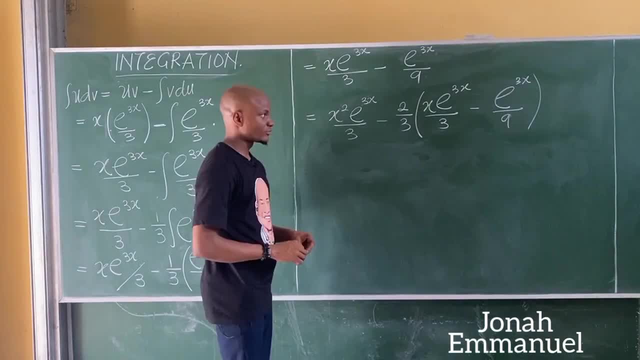 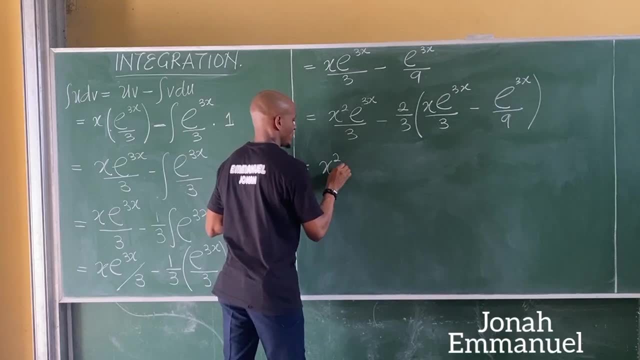 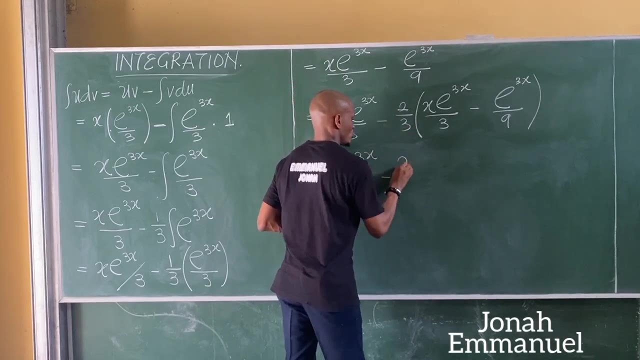 All Over Three Minus Exponential Three X. All Over Three X Square Exponential Three X. All Over Three Minus Two, But Three Times This. 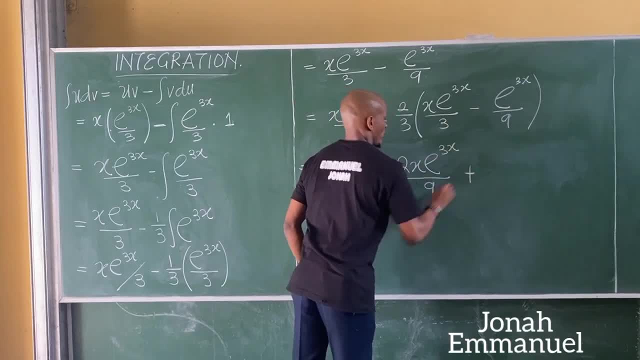 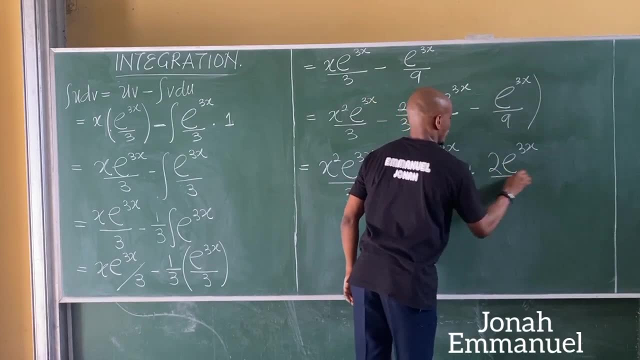 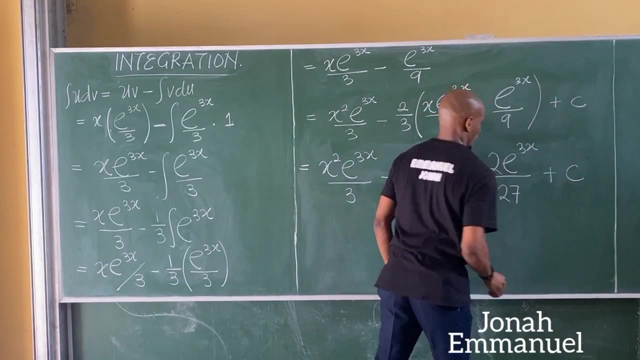 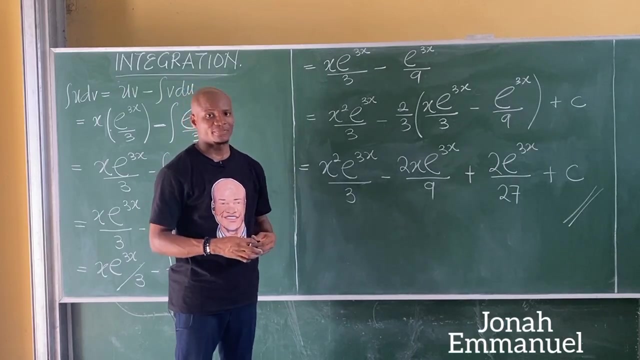 Gives You Two X Exponential Three X, All Over Three Times Three, Gives Nine. Next, Plus C Plus C, Which Is The Constant Of Integration. 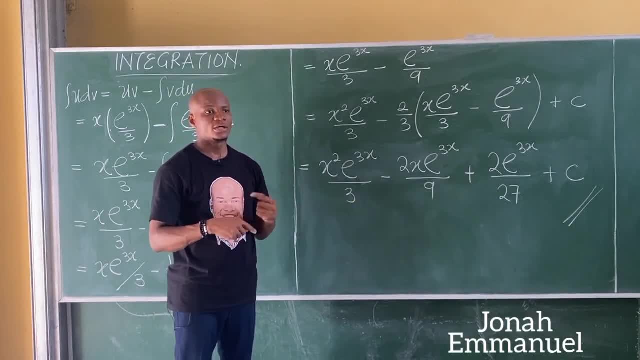 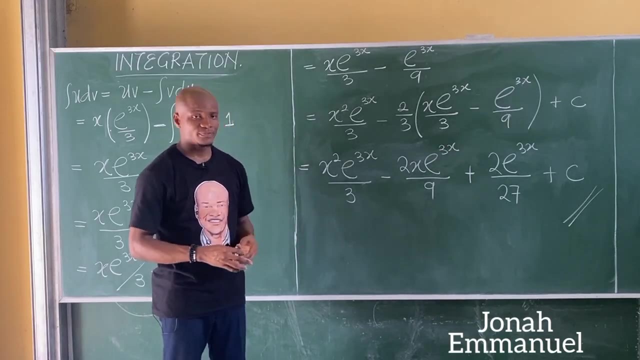 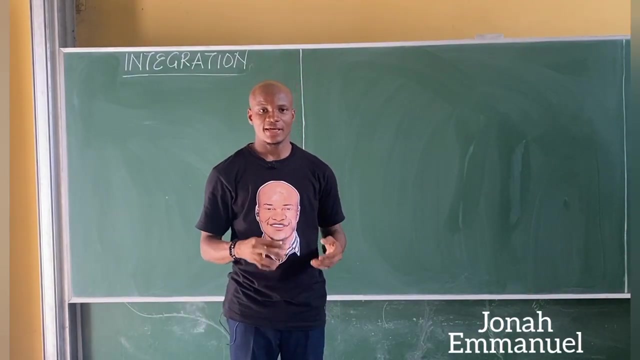 So Here Is Like Another Example Of Integration By Parts. For This One, Now Observe That For This Example. Let's Take Another Example Of Integration. 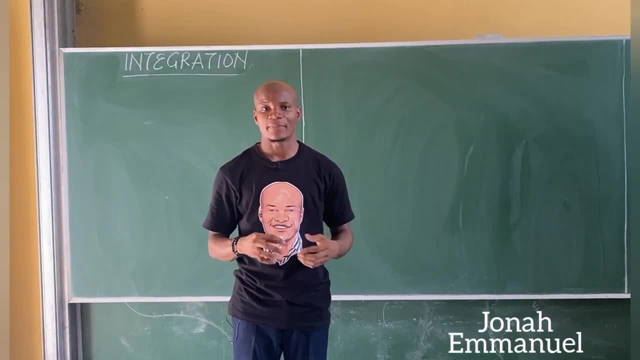 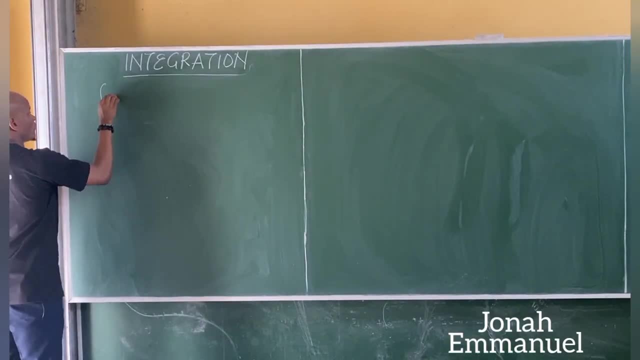 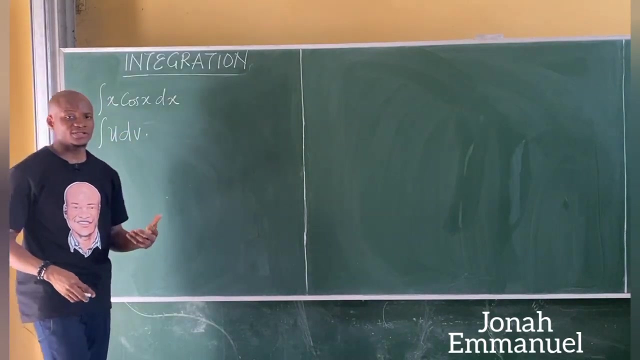 By Parts. So Let's Take Yet Another Example Of Integration By Parts. So In The Previous Example We Looked At Something Of This, But The 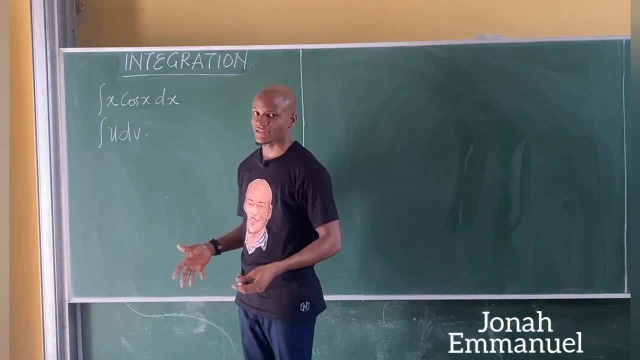 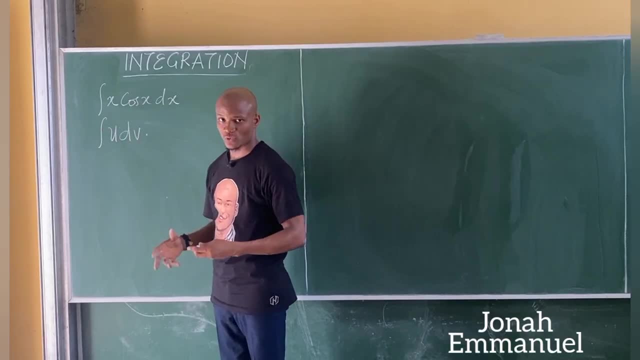 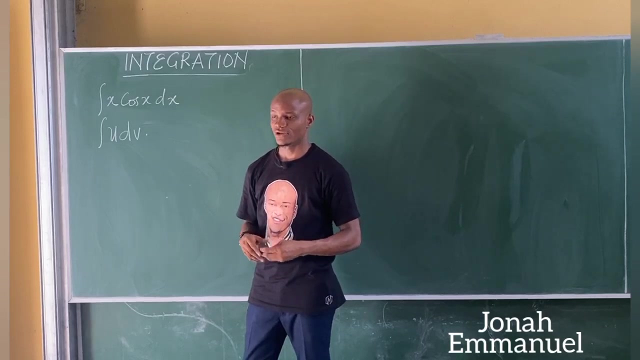 Question: Is This In Question Involving Integration By Parts, Does It Mean That You Is Always Equal To The First Term And Then The V? 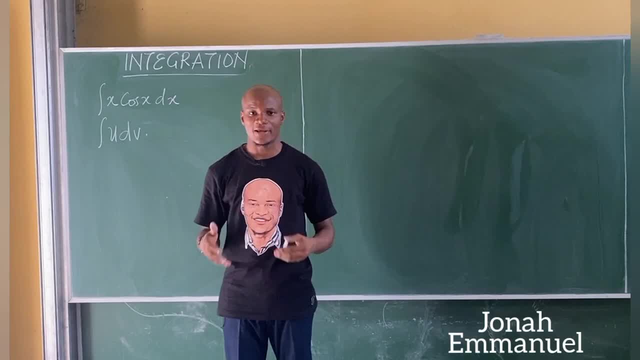 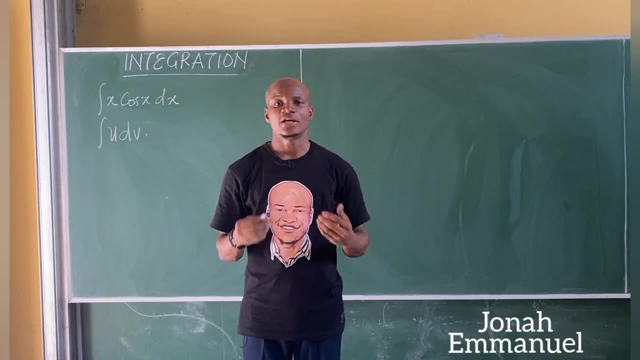 Equal The Second In Which They Are Placed. You Have The Same Result. So How Do We Know Which Term In Any Question Involving 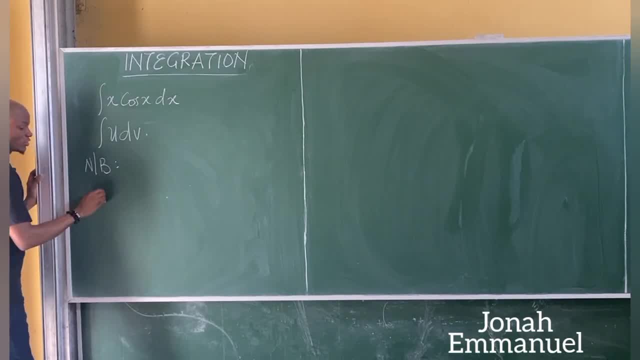 Integration By Parts. How Do We Know Which Is Equal To The Parts Of The Form Of The Function? So If I See In Class We 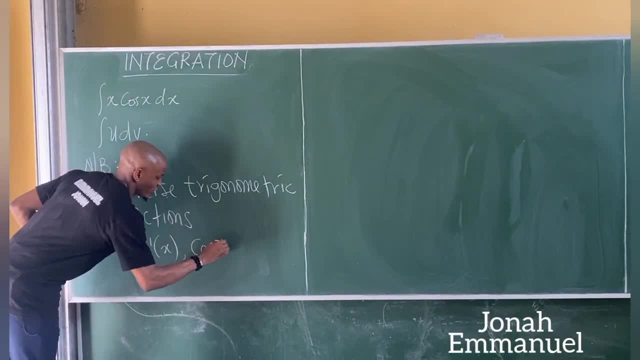 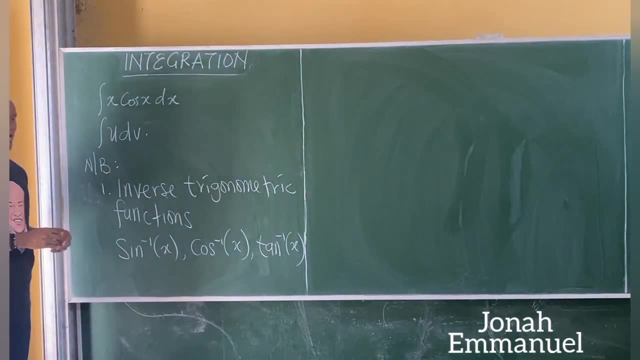 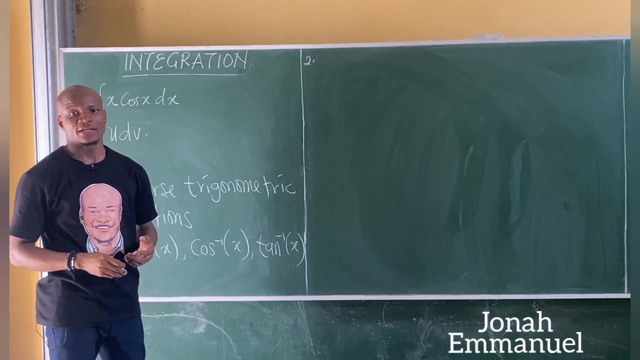 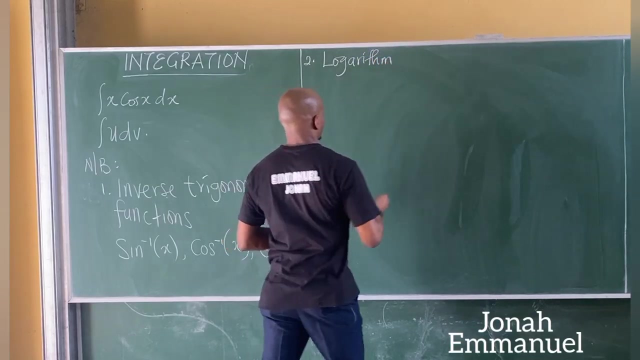 Will Make Functions. Always Take Them As You Example, If You Okay. The Second Kind Of Text To Take As You Are The Logarithmic Functions. 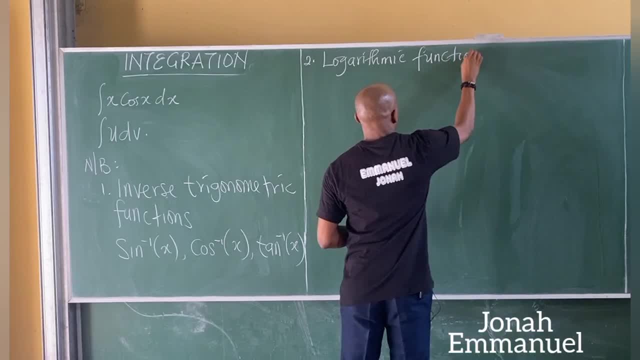 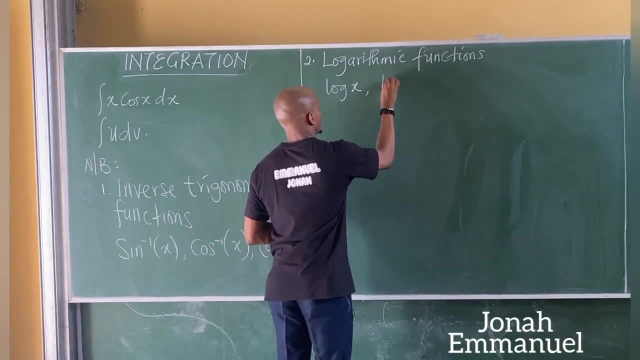 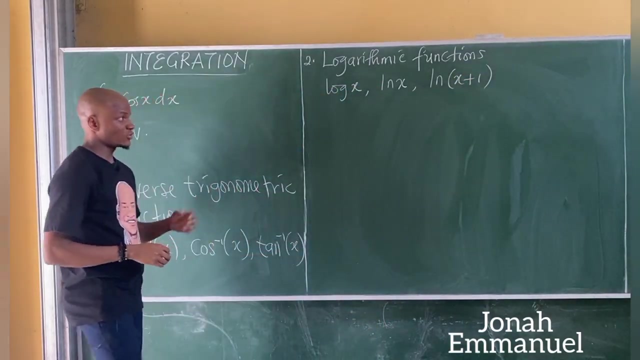 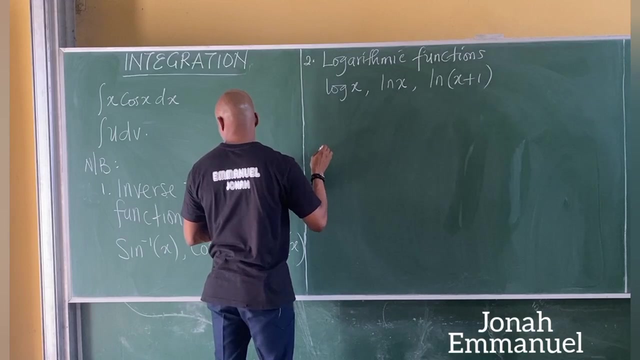 All Right, So You Is Always, Most Of Times, Used As Logarithmic Functions. Examples Of These Are Also This, Also Another Set Of Functions- We. 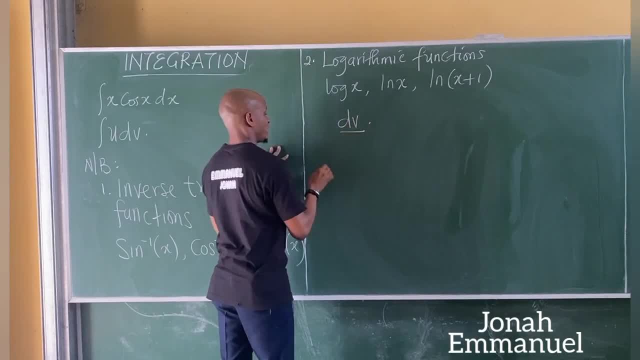 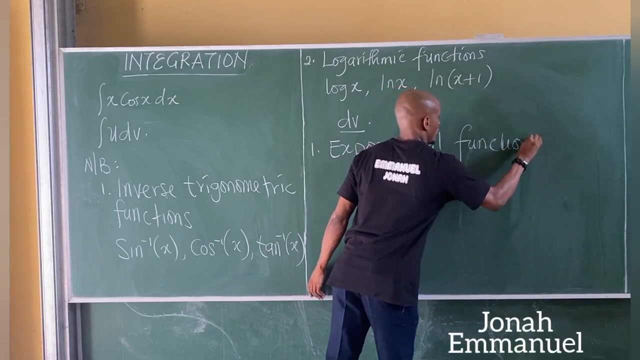 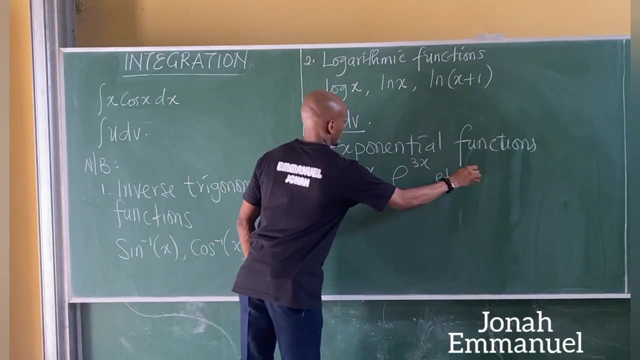 Take As You Also, When It Comes To The V, The V For The V, The Kind Of Functions Take Exponential Five, X Or Perhaps. 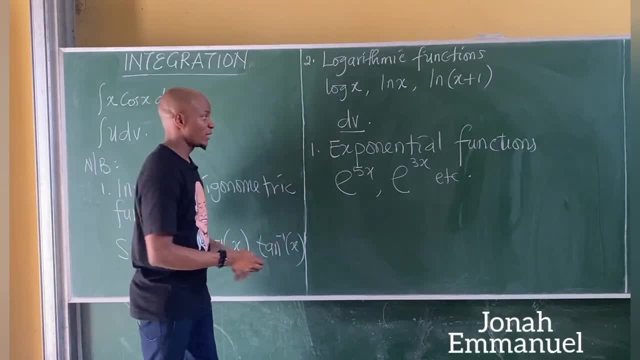 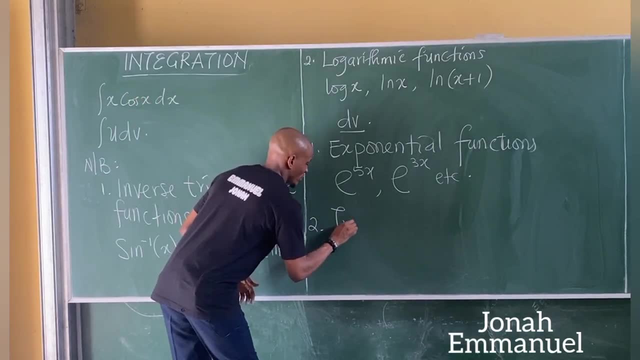 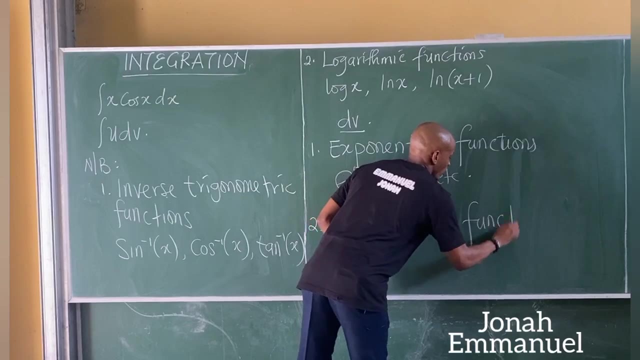 Exponential Three, X, Etc. So Exponential Functions Are Usually Taken As The V, Advanced Of Functions, Usually Taken As The V Are The Three. 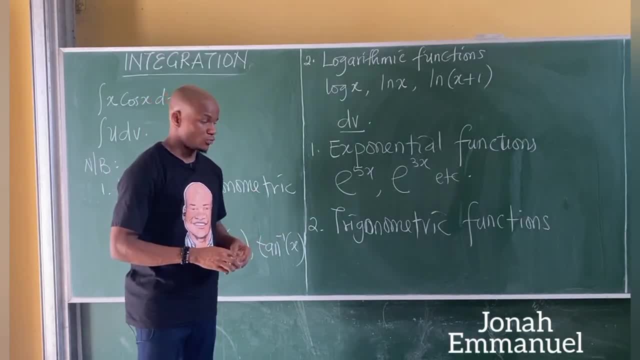 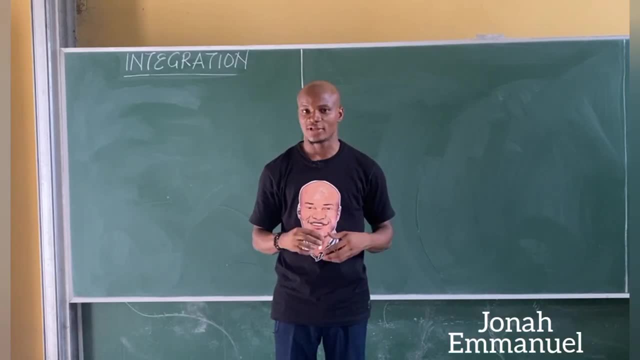 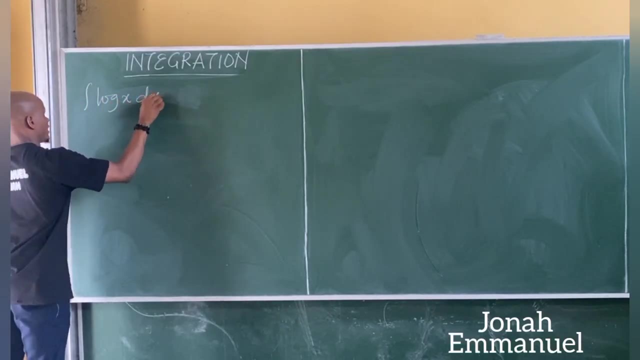 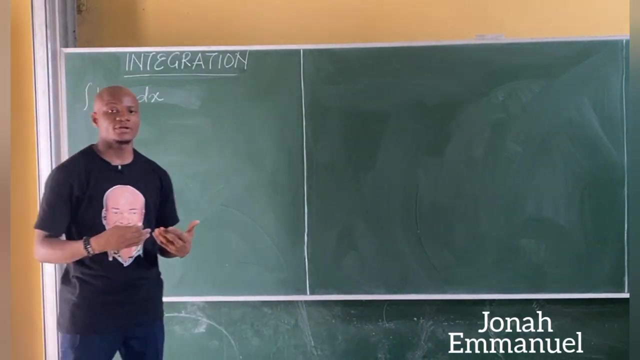 Functions As The V, All Right, So We Use This To Solve Some Problems. Let's Look At One More Example For This Class. Let's See: 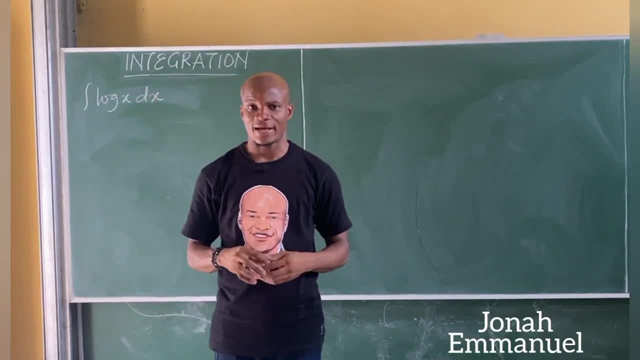 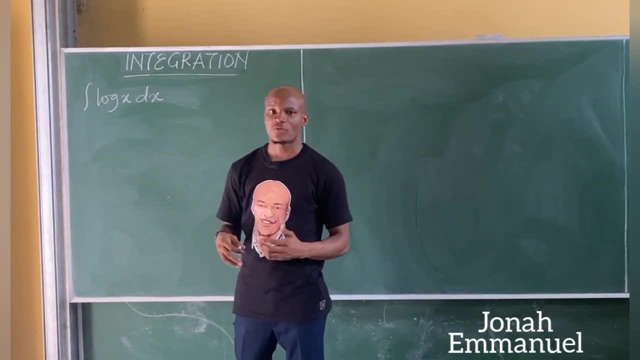 We Ask To Multiply, But In This Case I'm Having Just Log X And There's No Second Thing. Now, If I Have A Log X, 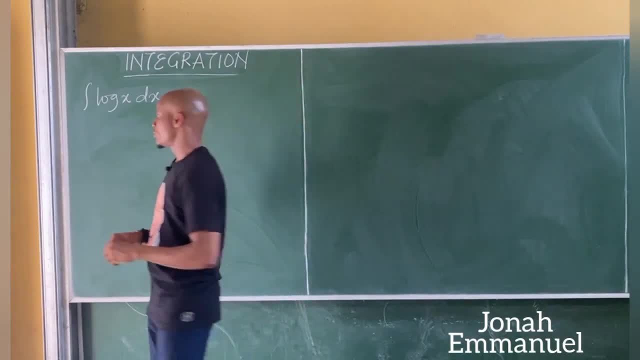 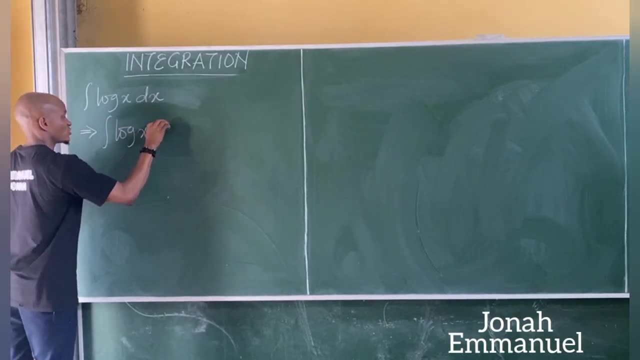 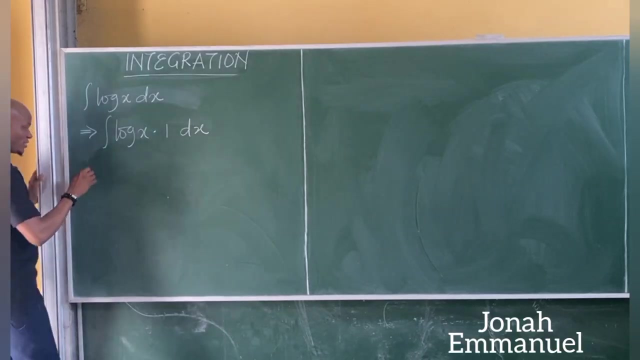 Question: Is This Log X? Will It Same As Same Integral Log X Times? One Of Course The X, So I Will Express This In This. 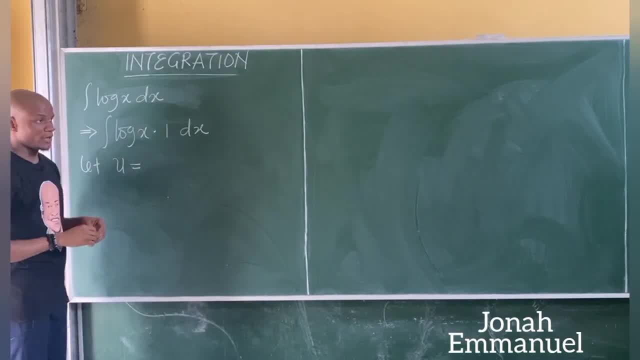 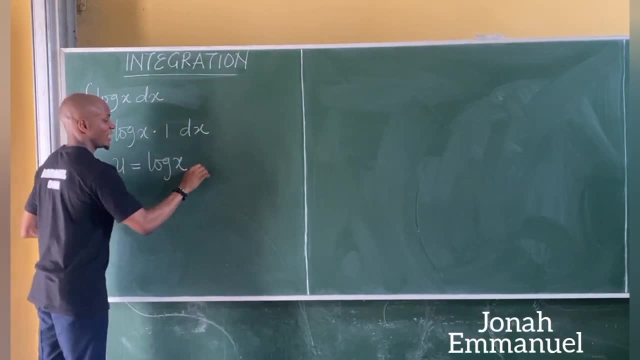 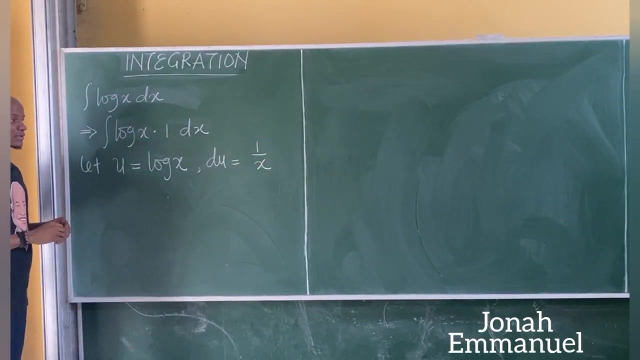 Form, And Then, Obviously, The V Becomes One Right. So Case I'll Have That The U Is Equal To, If I Differentiate, Log X: 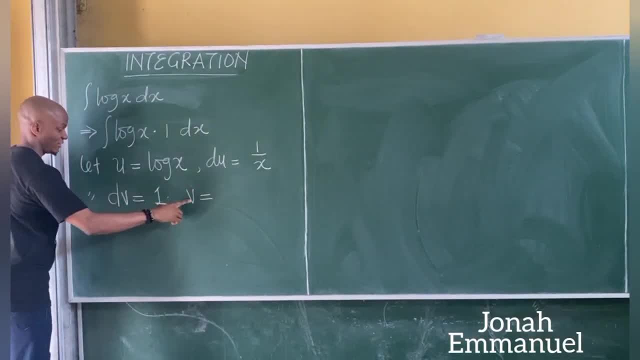 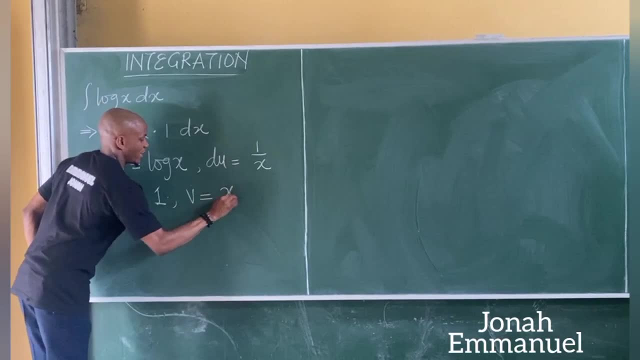 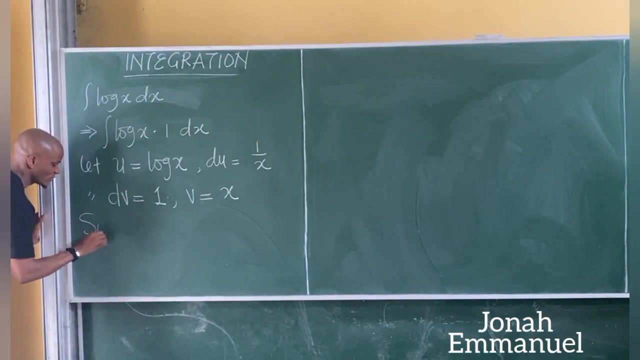 I'll Get One All Of X. Next, Let The V Be Equal To This One Of X. Substituting This Value. Substituting This Value. 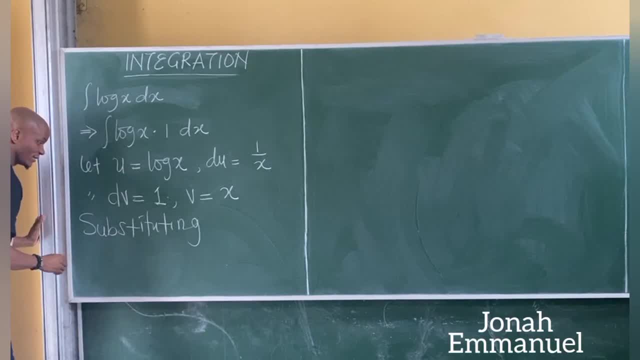 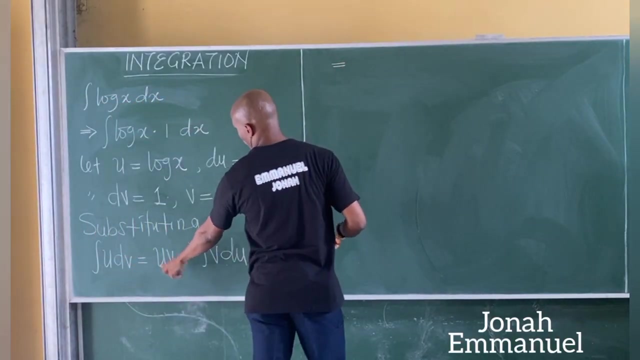 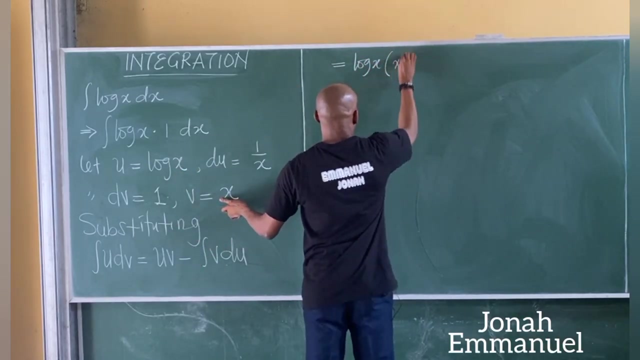 Into My Equation. I'll Have Instead. The Equation Is: Integral Of U In V Is Equal To U V Minus Integral V The Value Of. 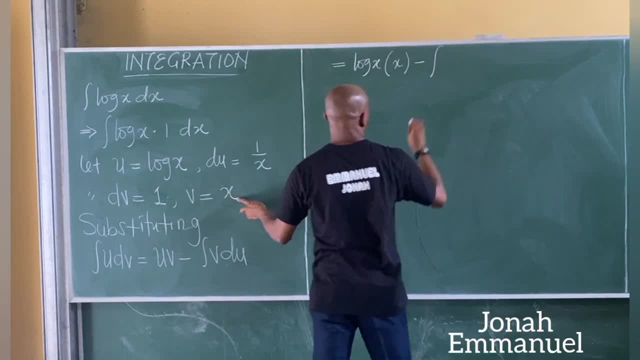 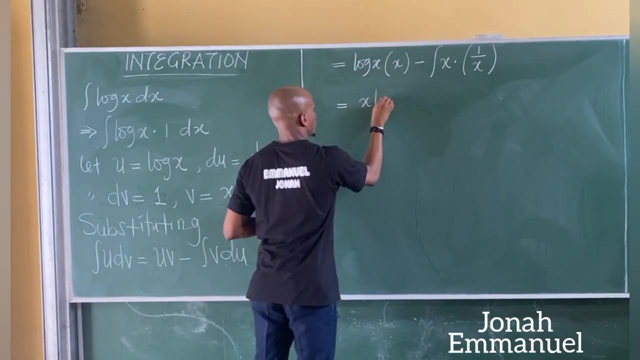 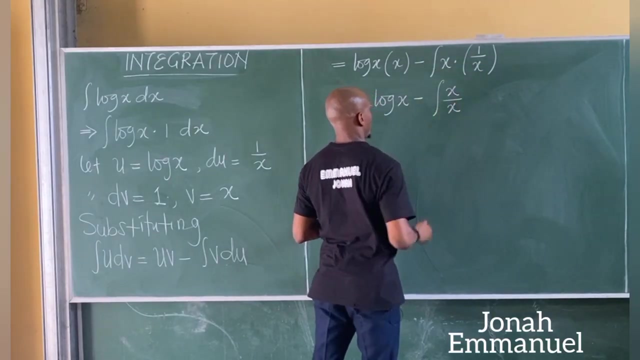 V. Here Is X Minus Integral V. V. Here Is X Dot The U, The U. Here Is One All Over X. So I Have 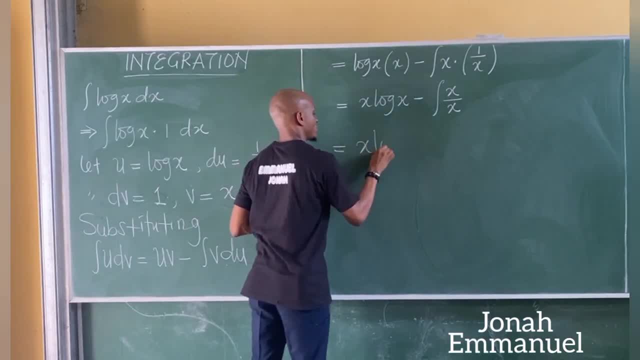 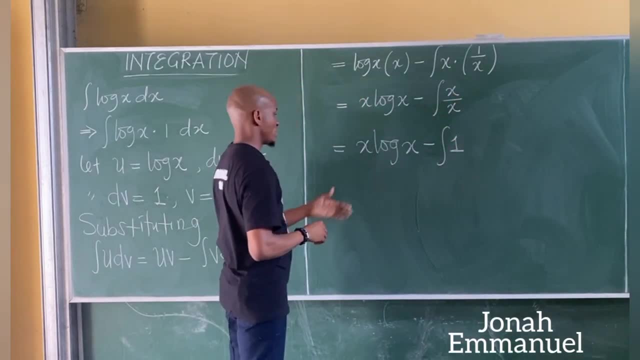 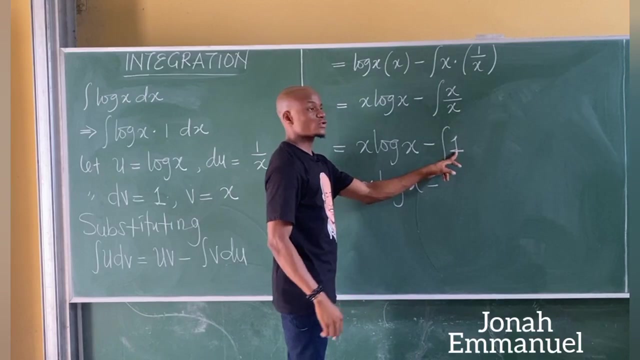 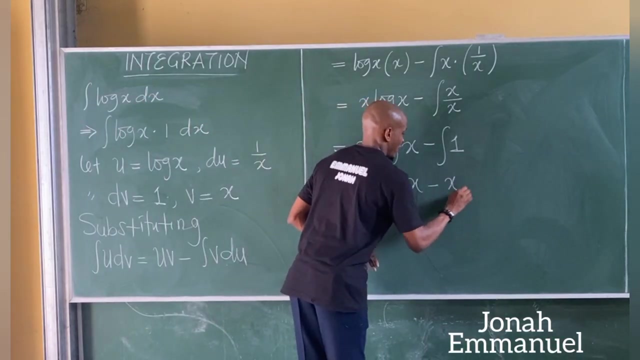 This: If Is Equal To X, Log X Minus X Over X Obviously Gives One All Right. If I Walk On This Now, This Is: 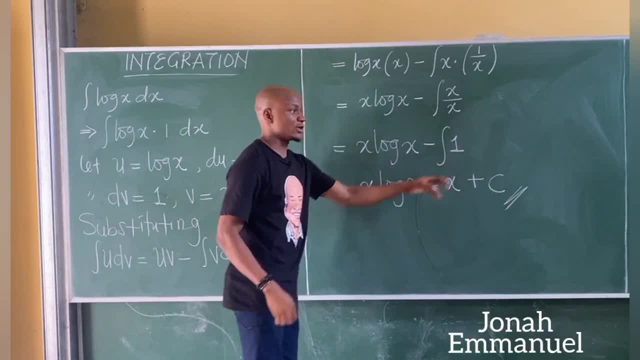 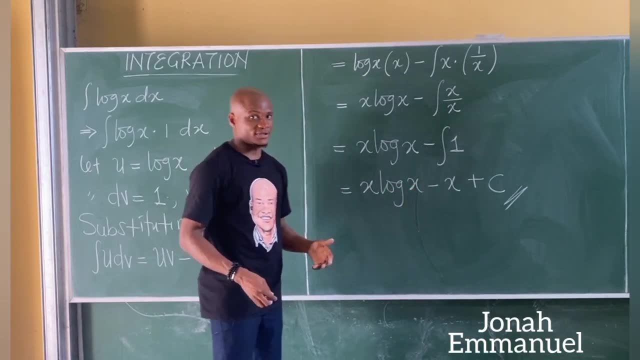 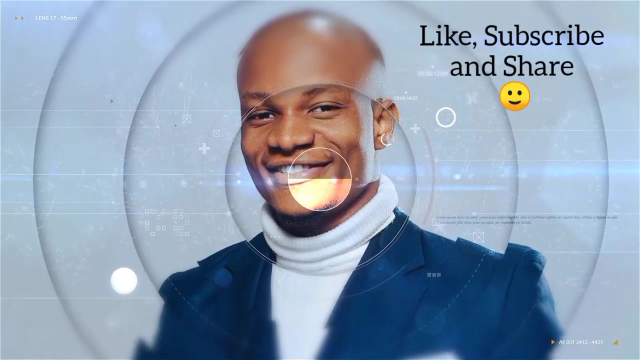 Going To X Log X Minus X To Give X, So Having X Log X Minus X Plus C, Which Is Your Constant Of Integration.